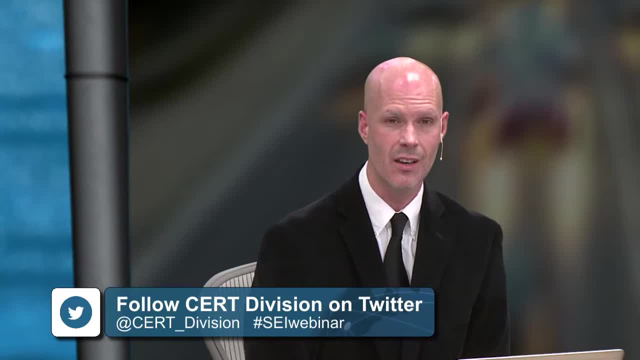 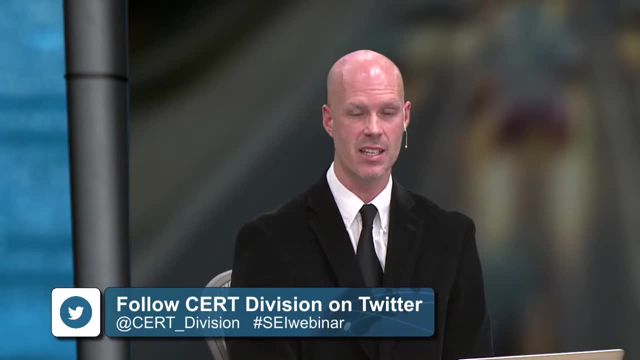 to be sure to follow at CERT underscore division and use the hashtag SEI webinar. Once again, it's CERT underscore division with a hashtag of SEI webinar, And now I'd like to introduce our presenters. for today, Dr Mark Sherman will serve as our. 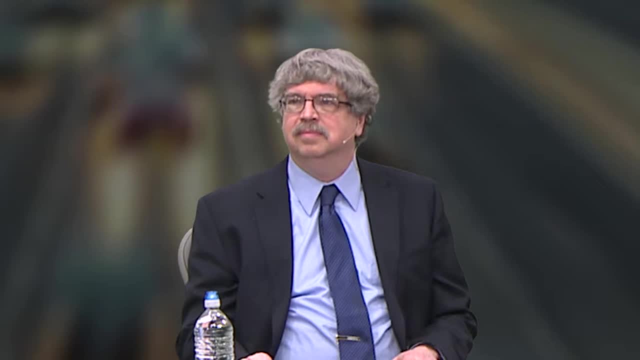 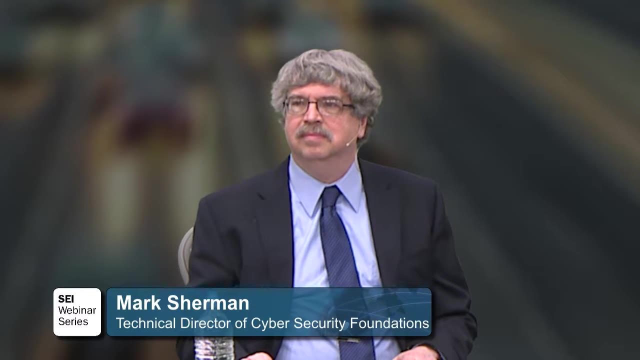 facilitator and also as a presenter today, and he is the Technical Director of the Cybersecurity Foundations Group at CERT within CMU's SEI. His team focuses on fundamental research on the lifecycle for building secure software and on data-driven analysis of cybersecurity. 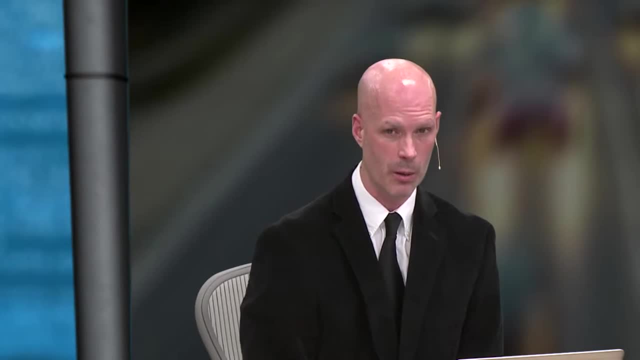 Before joining CERT, Dr Sherman was at IBM and various startups working on mobile systems, integrated hardware, software appliances, transition processing languages and compilers. He has published over 50 papers on various topics in computer science. I'd also like to introduce Mr Chris Vlasic. Chris will give our keynote talk today. 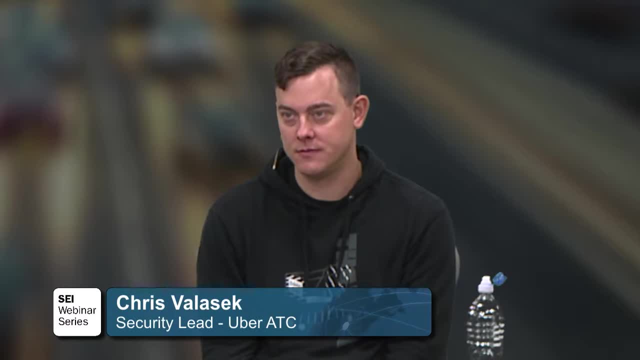 And Chris is the Security Lead at Uber's Advanced Technology Center, which is in Pittsburgh. He's regarded for his work in the automotive security arena And most recently, Chris was lauded for his remote compromise of a 2014 Jeep Cherokee, whereby he and his research partner. 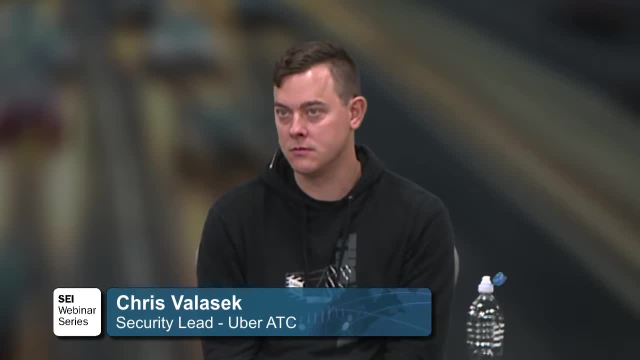 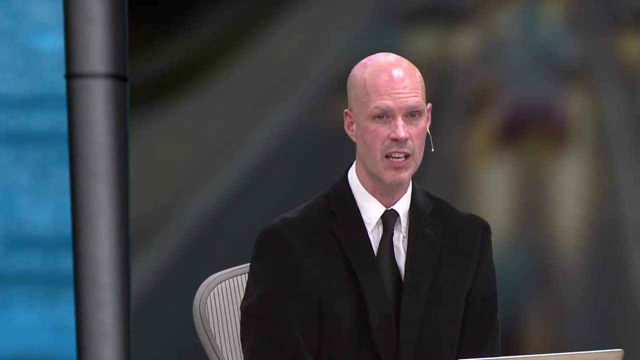 obtained physical control of the vehicle And he's also the Security Lead at Uber's Advanced Technology Center, which is in Pittsburgh. Vlasic specializes in reverse engineering and exploitation research, And Chris has a BS in computer science from the University of Pittsburgh and is the Chairman of SummerCon. 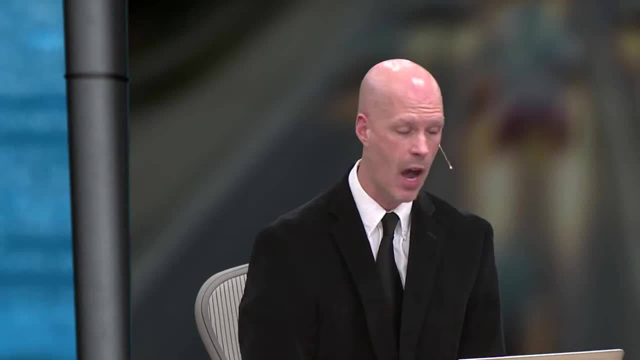 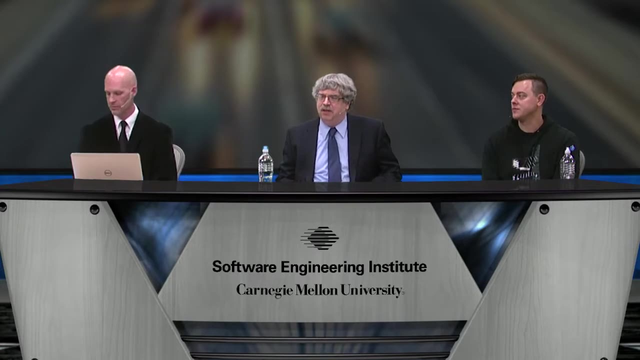 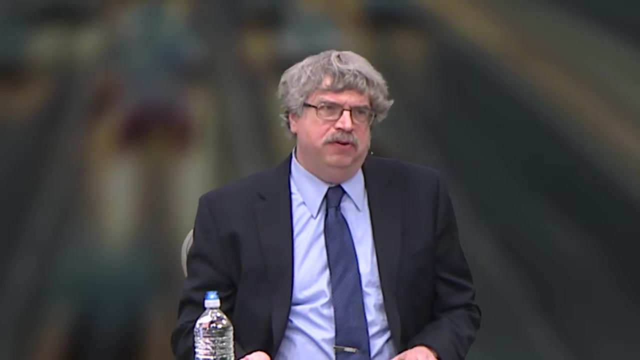 America's longest-running hacker conference. And now I'll turn it over to Mark Sherman. Mark, Chris, welcome, Thank you. Thank you, Shane, And welcome everybody to this webinar. I appreciate you spending several hours of your day with us, And we're going to talk about a very important. 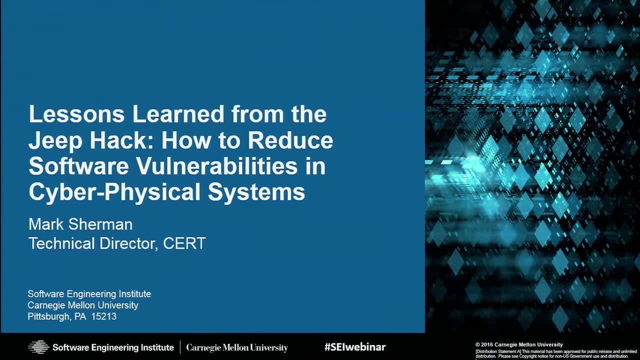 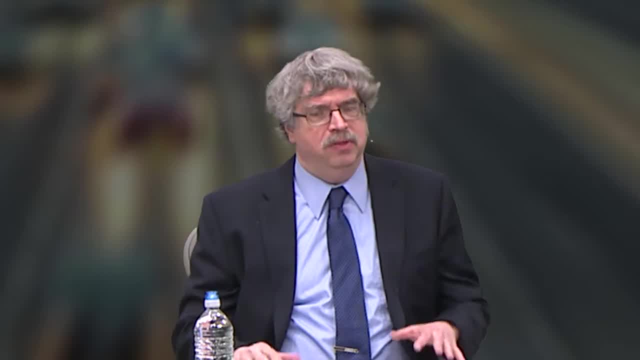 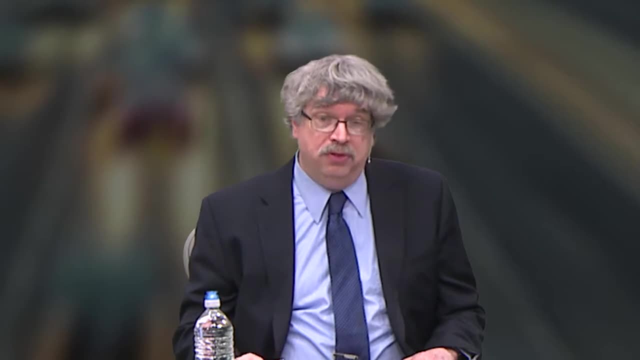 topic about the risks that are involved in or emerging on, cyber-physical systems, The attacks on IT systems, whether they're the target system in retail. what happened to office personnel management in the federal government? Anthem Health in healthcare, Sony in entertainment- these have all been IT-related that released information that was harmful. 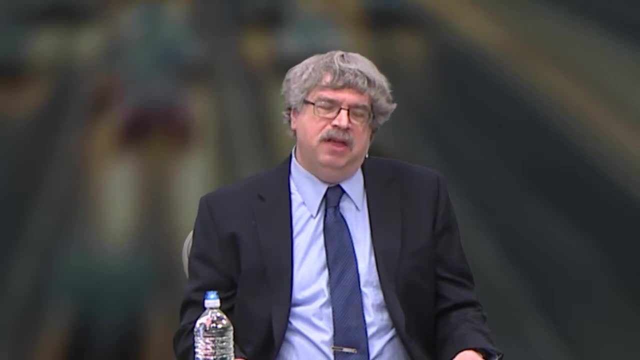 to the organization and individuals. What's happened now is that this is moving into the cyber-physical space as well. So we've seen steel furnaces in Germany attacked. We've seen hotel locks being able to be disabled, the electric grid in the Ukraine. 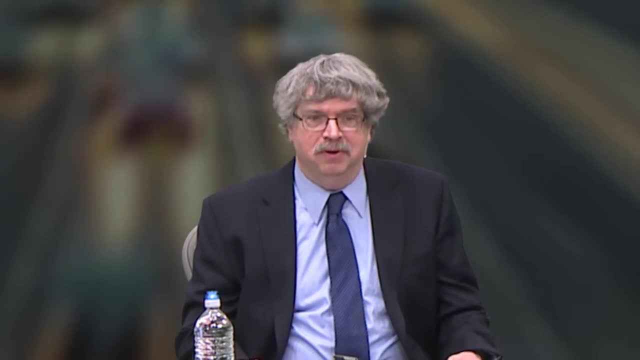 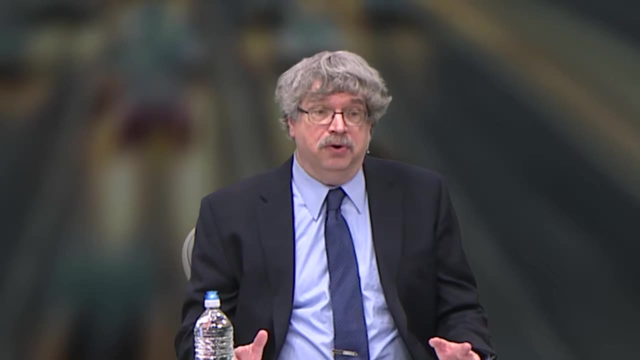 insulin pumps have been disabled and, of course, the very popularized Jeep remote control. But when these kinds of events occur, we can get physical damage that causes problems to real people. I'm going to share with you that today we're going to see some of the latest developments. 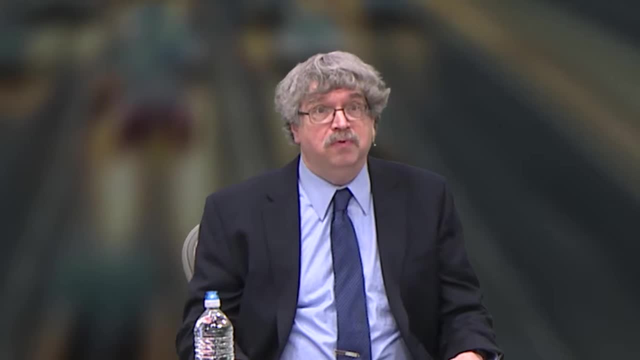 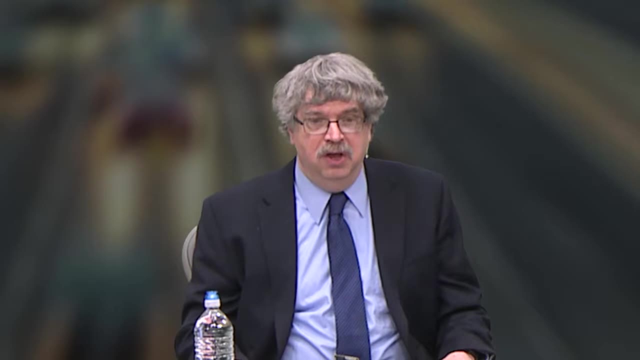 that we've seen, that have been changed and have taught people as much as death, like some of these medical devices. It's important for us to figure out how to build systems that are more resilient to attacks, to eliminate the vulnerabilities, in order to have a better 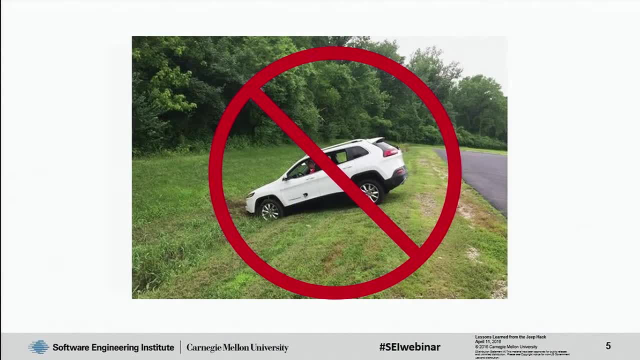 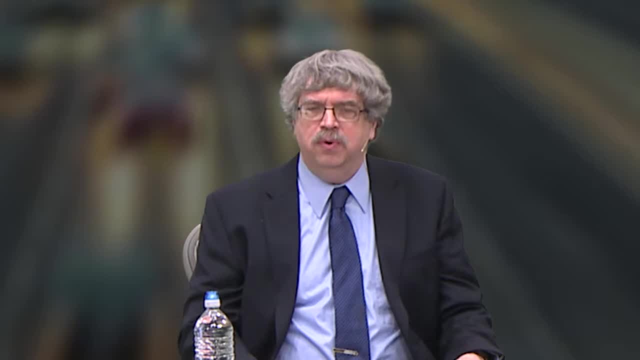 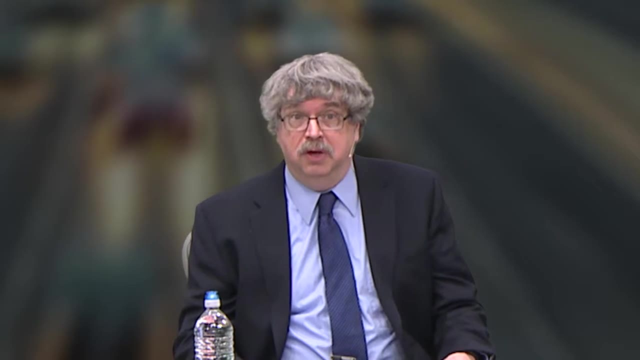 environment. Ultimately, what we are intending to do today is basically not be the next Jeep. We have learned many things from these various events, that many of what's going on, the vulnerabilities that are there are well understood and the ways to avoid them are well understood. 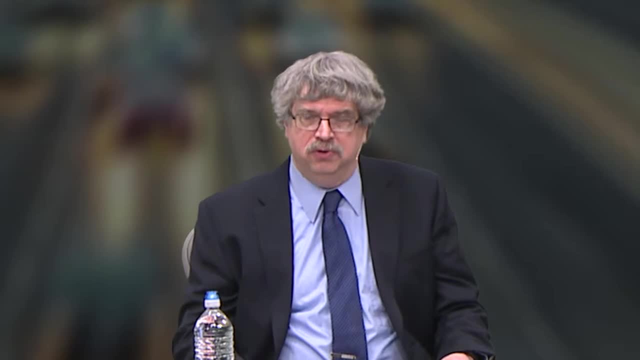 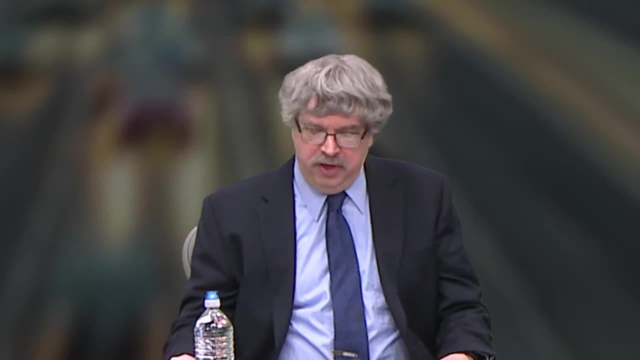 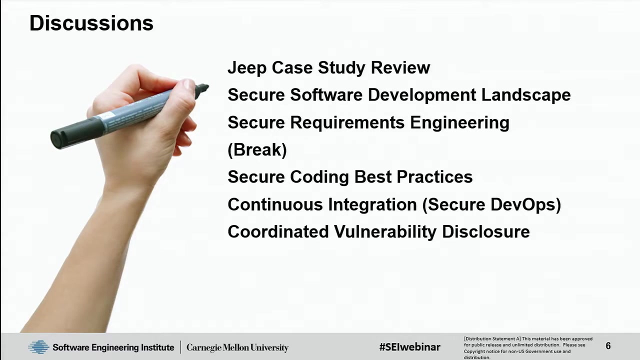 That if we apply what we already know about building secure systems, we can make the cyber, physical world a lot safer than it is today. In order to do that, we're going to go through a range of topics that will help understand better how to build these kinds of systems. 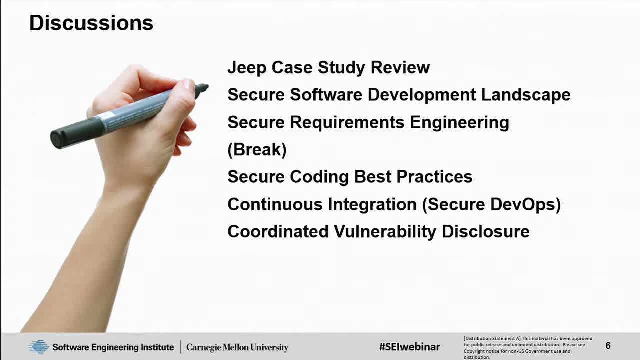 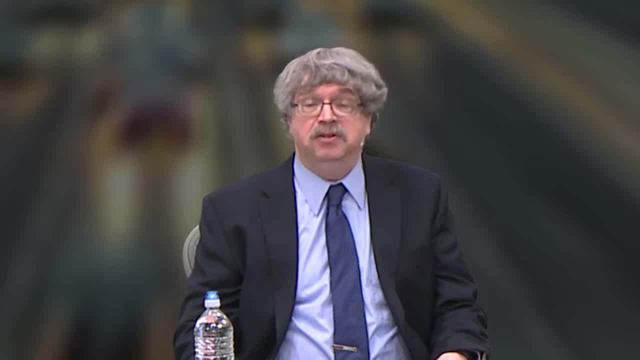 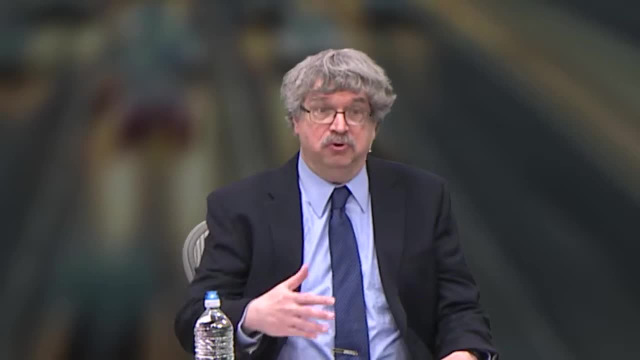 Of course, what one starts with is analyzing in a little detail how some of the vulnerabilities have already been exploited. We'll start with Chris's help on the Jeep case study. We will look at some of the details of how the Jeep was able to be controlled remotely. 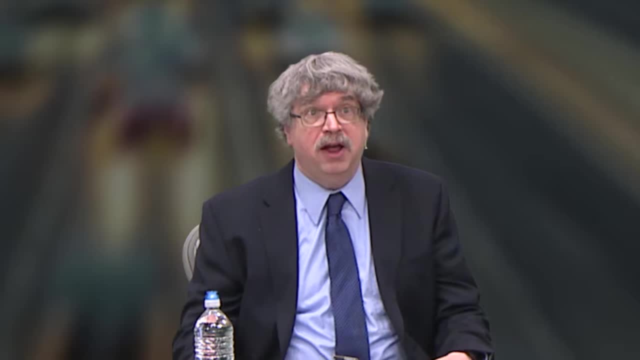 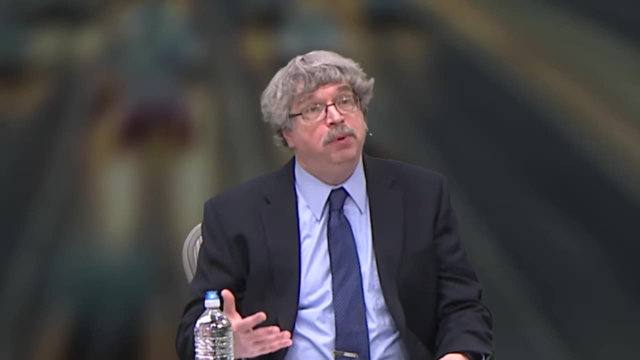 From that we'll take a look at how one builds secure software and how that would have better enabled the Jeep to be resilient to this. We'll give an overview of that And then delve into it. In a couple of the specific topics we'll focus a bit on requirements we'll discuss 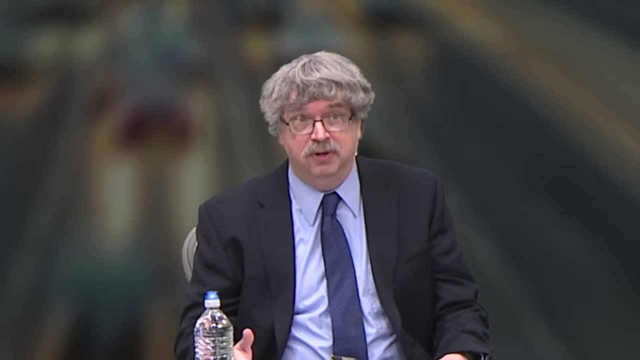 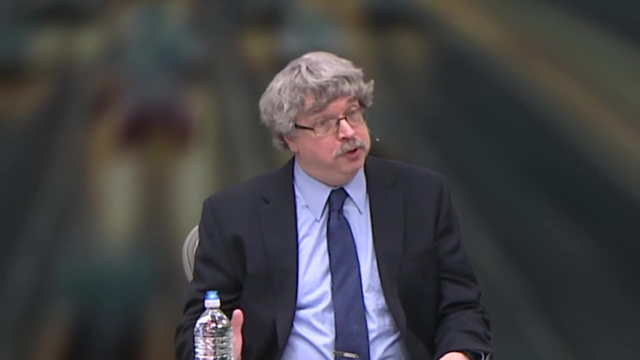 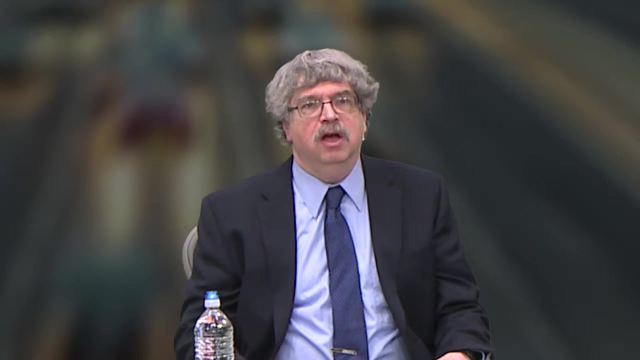 a bit about how one actually does the programming of these systems. we'll talk about how one automates this whole process in order to rapidly bring forth better software. and, of course, breaches will be inevitable despite our best efforts. So what is the best way to handle those kinds of events in order to minimize the damage? 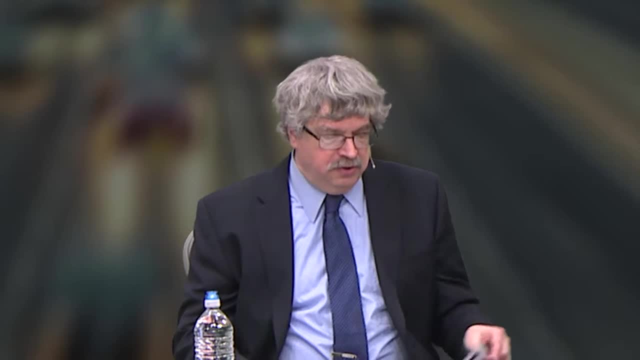 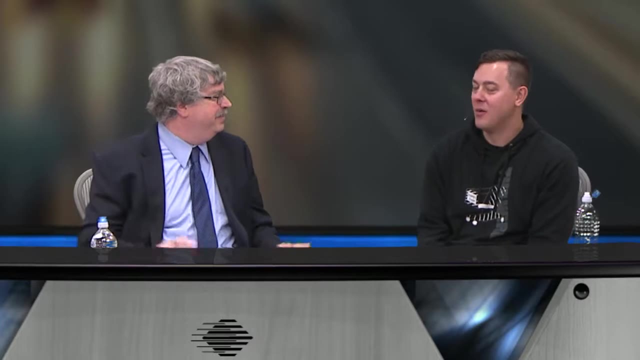 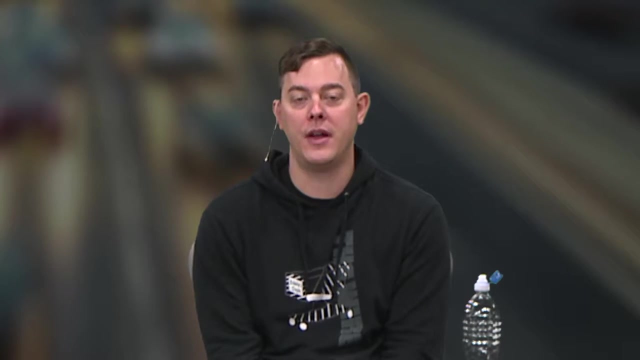 that might occur. So to start with, I'd like to turn to Chris. Let's have him discuss a little bit about what happened with the Jeep. How's it going, Mark? Good, Excellent. Well, I think many people have seen the Wired video and kind of saw us playing around with 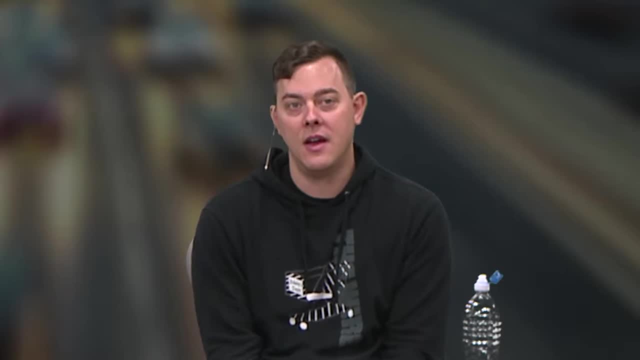 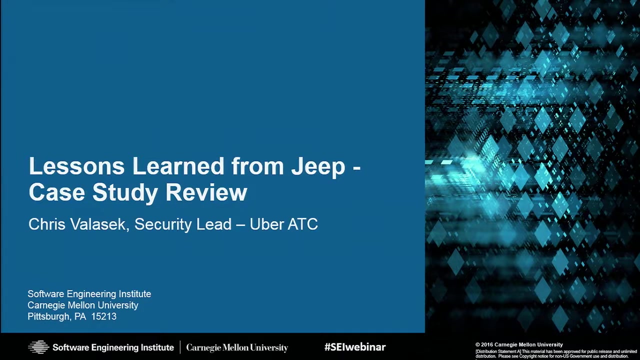 Andy and thought that was the extent of it. In reality, it was a year-long effort of analyzing these systems. Additionally, we released a paper a year prior that actually was a survey of 25 different automobiles. That paper was actually us looking for our perfect car that we thought we could compromise. 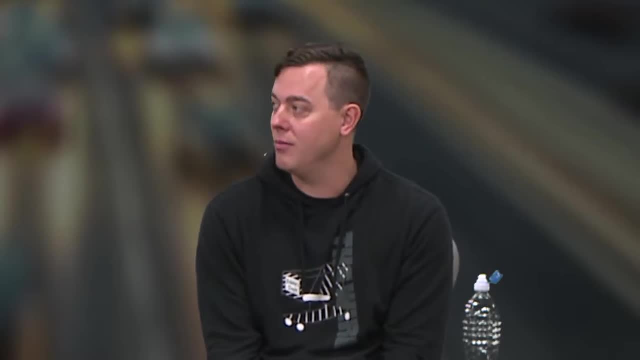 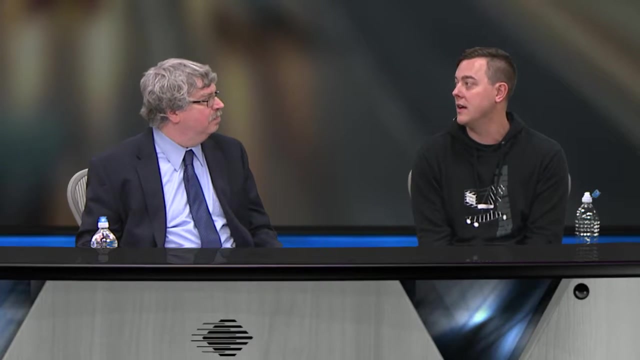 for physical control remotely, And the Jeep stuck out because it had a lot of external communications, such as telematics and Bluetooth and even in-car Wi-Fi. Additionally, there was no apparent separation between the systems that control things like steering and braking and acceleration and those items that were communicating with the 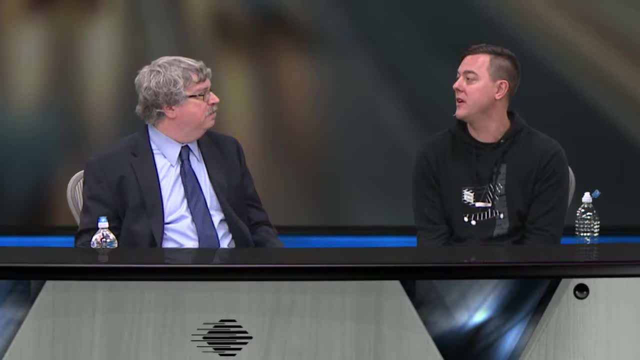 outside world. So we really- Yeah, Yeah, Yeah, We did this preliminary research to pick the Jeep as our target. That was our kind of first step in doing all this, and that will show you one portion of security that needs to be considered when designing these things, right. 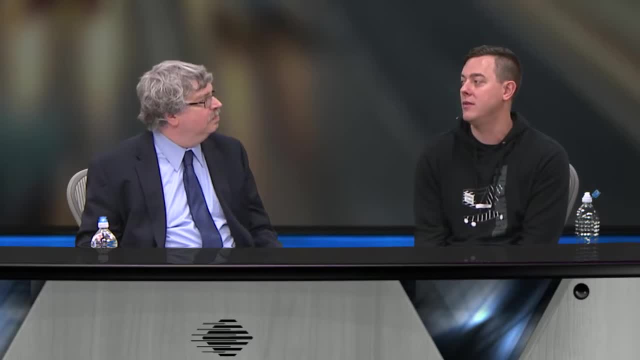 You need to understand that if you're going to have it communicate with the outside world, what can it touch directly or indirectly? Many times people will assume, just because two systems are on two physically separate circuit boards, that they are actually separate, when indeed they're not right. 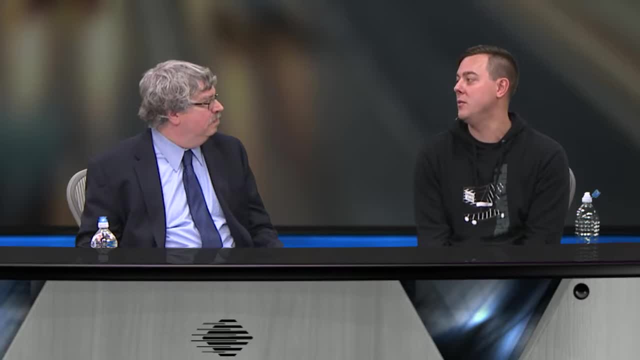 You can have a serial line, for example, have these two things communicate together, Even if they're not made to communicate in the fashion you've designed them for. people like Charlie and I think about things differently. So we're using those systems to perform physical control when I think. many times people thought that wasn't the case. Yeah, I saw a study that came from the Department of Transportation in, where they were doing an analysis of how you get into cars and at one point one of their researchers had counted up that there were 50 different antennas. 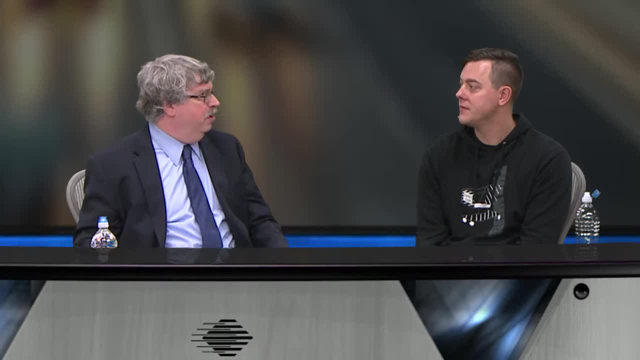 They were a bit encompassing of that inclusion. So your phone that you kept in your car they also counted in that. but they also were looking at that. Did you see that as a major issue as to how the number of entry points in? 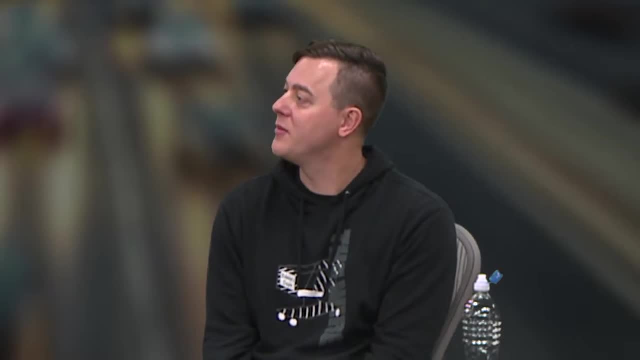 Yeah, absolutely. I mean even things such as your tires have radios in them, right? Yeah, Because after a certain year it's mandated that you have to have tire pressure monitoring systems, So there's communications coming from all over. Luckily for us as consumers, it's pretty transparent. 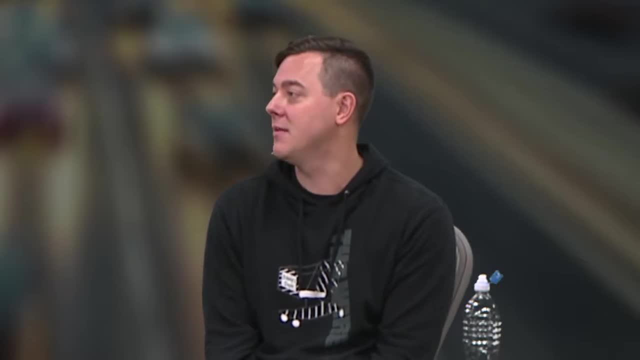 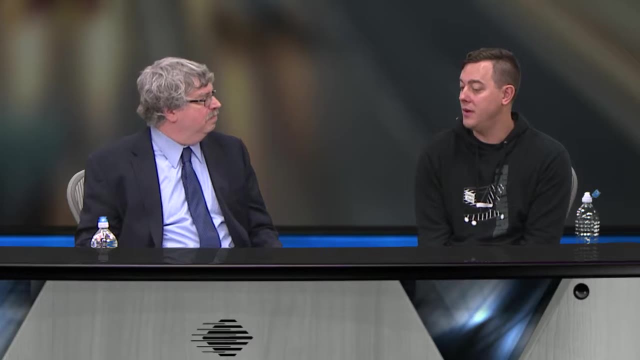 I like that, I like the technology, But you obviously need to be thinking about security when you have external communications. A lot of these attacks were possible because it was internet-connected devices that were linked up with other control devices that were, to be honest with you, designed before. 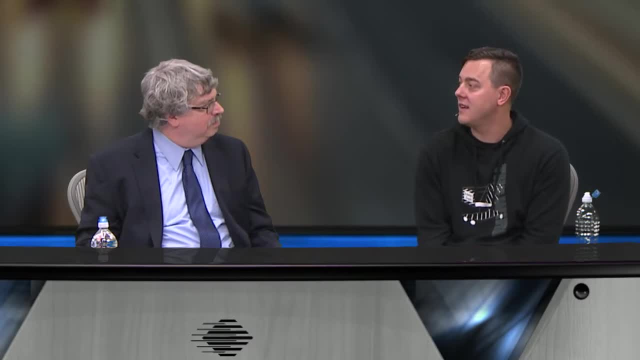 connectivity and security were even a thought. The CAN standard was developed by Bosch in the late 70s or early 80s and they were for really automated control systems that were self-contained, And this was before you were giving it the cellular modem or Bluetooth connectivity. 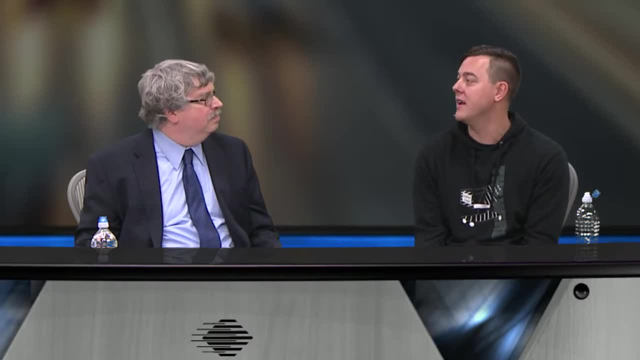 So they're not designed to be as resilient to replay attacks or have any level of authentication built into them. This gets problematic, as you can see, when you have these internet-connected devices touching these things. So can you tell me the story? Yeah, 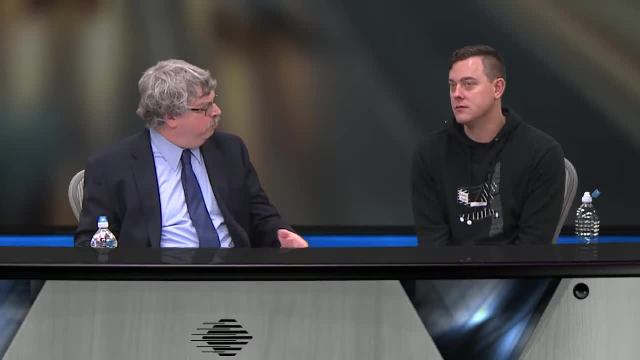 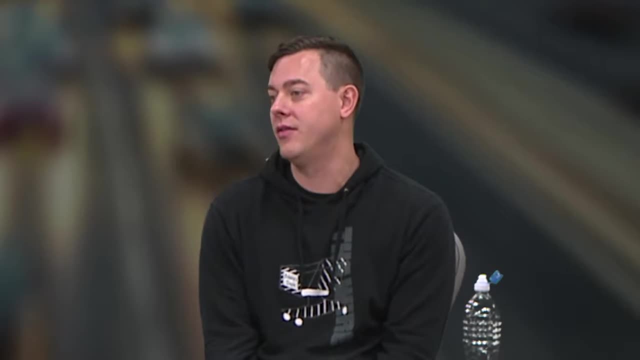 Can you tell me the steps that you took in order to get remote control of the Jeep? Yeah, There were a lot of steps, and any one of them could have- I don't want to say prevented it, but would have made it much more difficult. 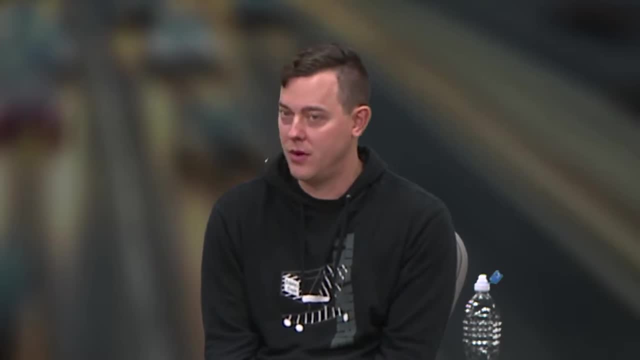 The first thing that we really did was that we understood Wi-Fi. Charlie and I were former pen testers back in our day, so we figured, if this car has Wi-Fi, we at least know how to look at that. That's normal to us. 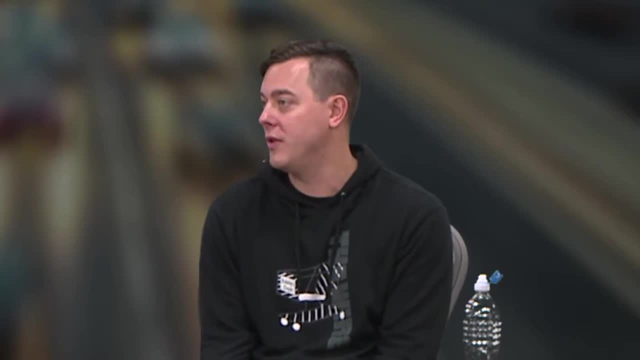 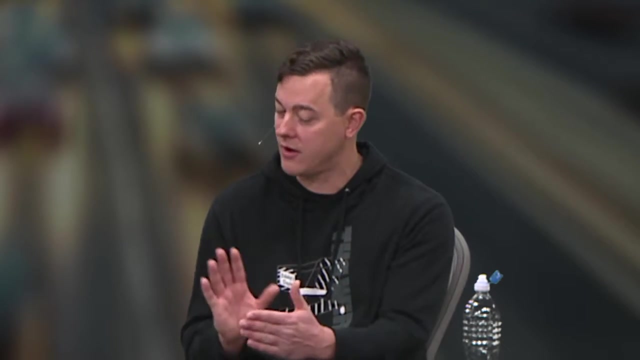 It's just a computer internet connection. So, lo and behold, we found that indeed it actually had a lot of ports open, And these ports were accepting unauthenticated communications that would pass user-inputted data to scripts that they use on the actual head unit of the vehicle. 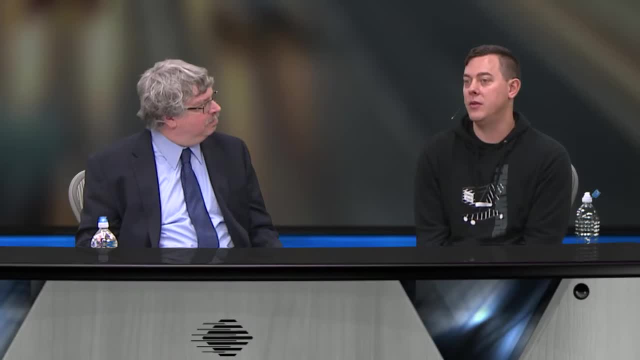 It was Harman Kardon who produced this head unit. It was interesting because we didn't think there would be any open ports, because it should just be a router. But needless to say, it was our first choice of investment, So yeah. 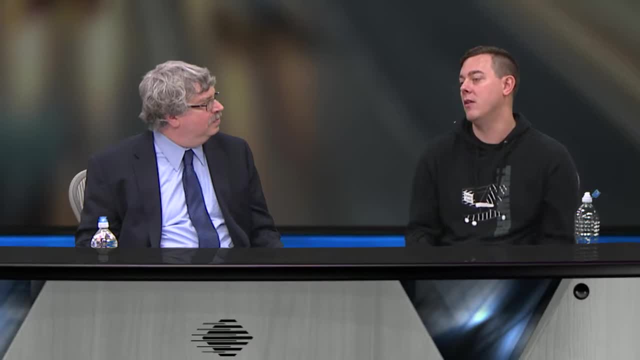 It was our first choice of investigation. At the same time, we were in parallel looking at how we could do cyber-physical controls of this vehicle. So when you have a car, you want to look at the type of messages it sends when it's parking. 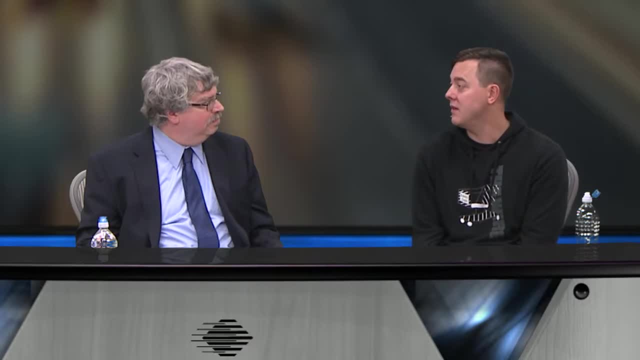 itself, or when it's putting itself into a maintenance mode for mechanics to bleed the brakes or things like that. So we were looking at these things in parallel as time went on, and this did take quite a bit of time to figure out. Early on we found that there were some scripts that had things like command injection, which 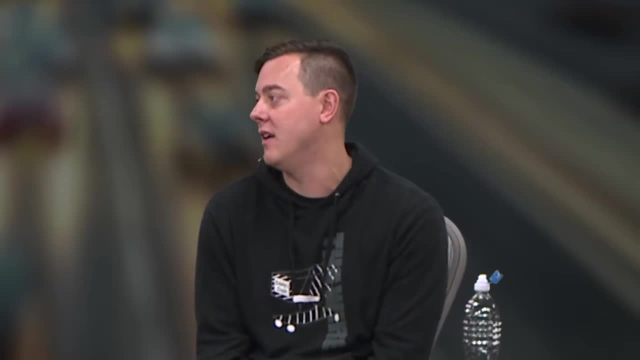 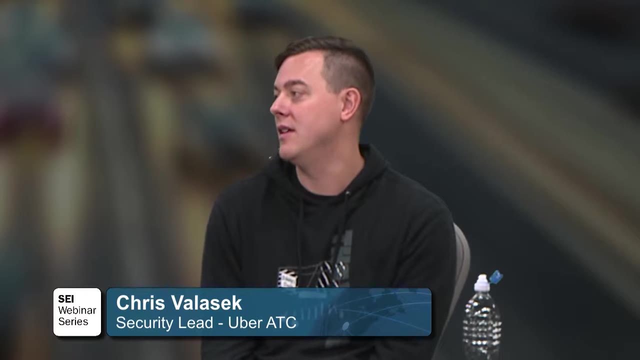 is pretty well known in web applications and regular user applications, but it just so happened that it was on an infotainment system in a vehicle. We realized, even after looking farther, that we didn't need to actually exploit one of these vulnerabilities with command injection because there was a script called execute. 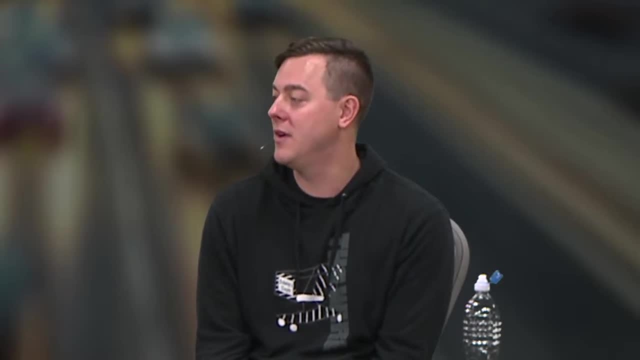 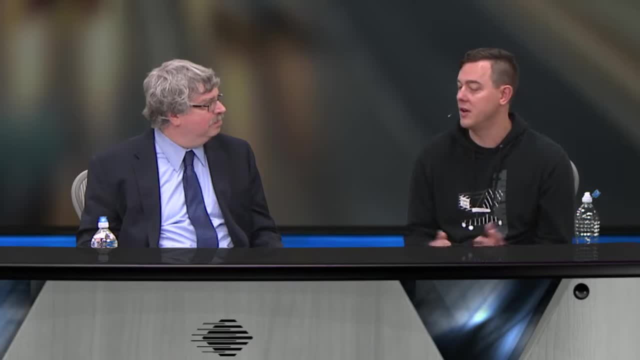 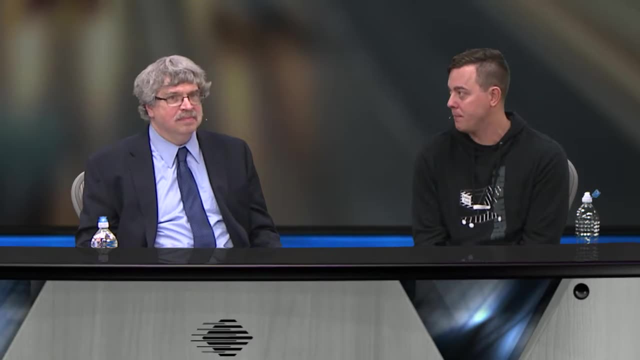 privileges on this infotainment system. You can imagine sitting down at your Windows or Linux machine and you have administrator or you have root privileges. You can do anything you want. That being said, that didn't mean that we could send messages out on the CAN bus, because 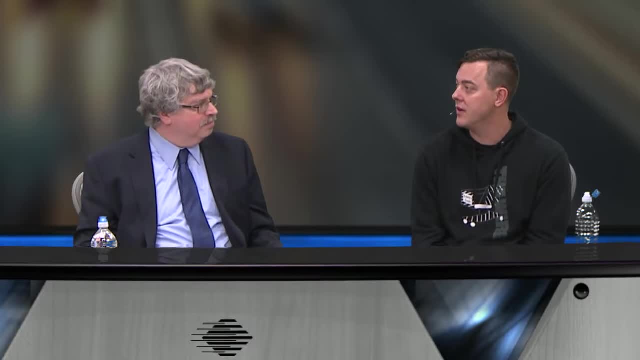 it wasn't designed to do that. There was actually a separate microprocessor that was used for that specific application. So our next portion- Mm-hmm time-consuming- of this was getting the firmware off the chip that was doing the cam controller work. 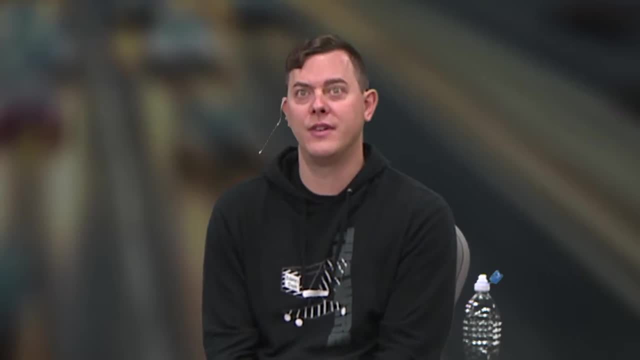 and figuring out what it did. This actually took us several months to figure out, because it's basically just a binary blob that you don't know anything about And you have to figure out exactly what it does. So we spent forever looking at this. 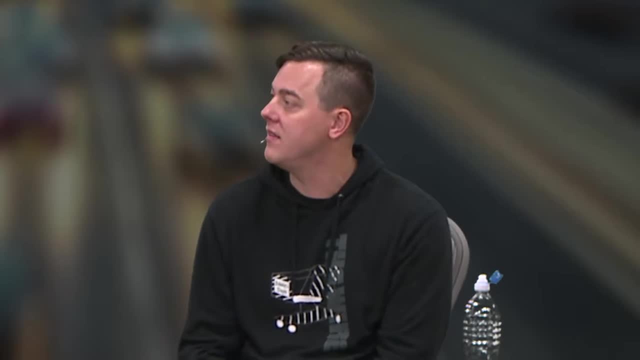 And we finally realized that, hey, this is where they send messages And these are how messages are set up in memory. If we could somehow alter this a little bit, then we would be able to reprogram the cam controller to have our own version of this code on there. 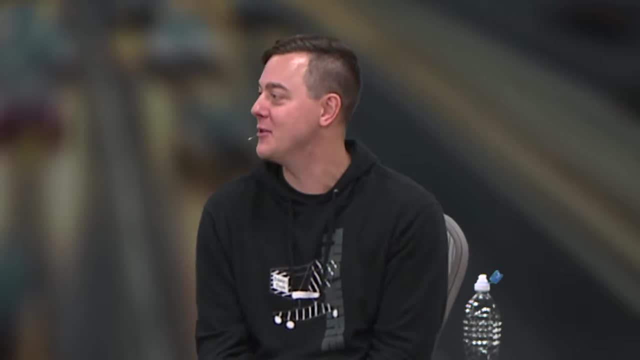 Remember, this is all binary. You're literally looking at hex bytes, right. It took a long time But we figured out we could actually do that. But we had no way to actually get it on the cam controller because the head unit was separate. 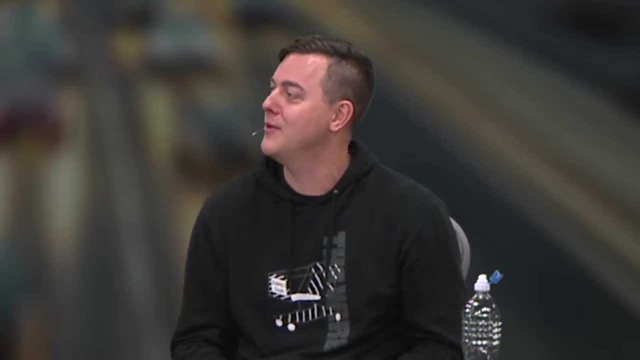 They were literally two different boards. There was an actual. There was an air gap in between the two. Fortunately for us, unfortunately for FCA, they were still connected by a serial line communicated by a SPI- S-P-I We found 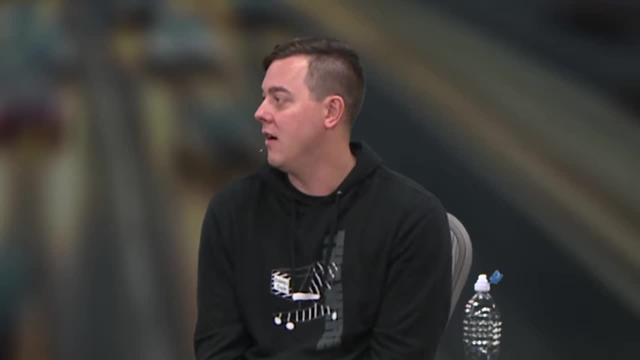 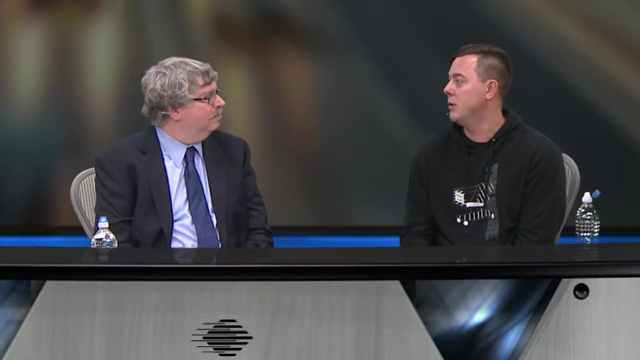 that there was no concept of code signing on these binaries that were getting flashed to these systems that physically control things, So we could alter the code to do what we want and then actually reflash the chip with a utility from the head unit to the cam controller. 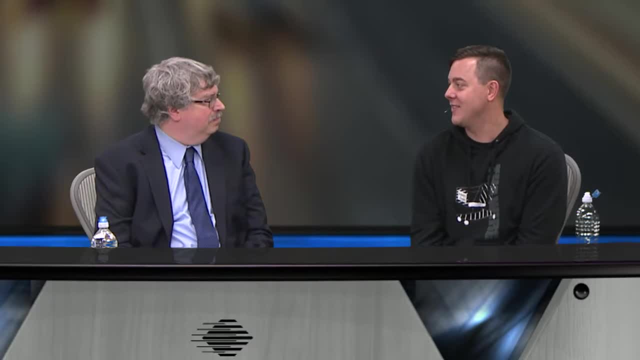 OK, Which was discouraging to see in something that should have certain levels of guarantee of code running it. They do a lot of testing in vehicles to ensure things like your safety belt works and the airbag deploys on time, But then there was no checks to see. 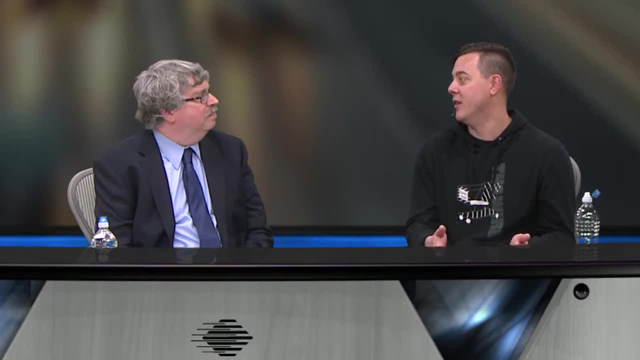 if the code running on that was actually their code, right? So that was the first concerning part. Even if we were able to do this, which we were, there was no direct method. We had to do it from the head unit to the vehicle. 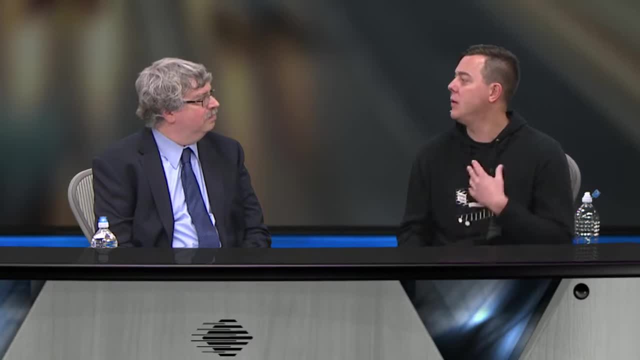 where you could say: here's a CAN message, send it out Any one you wanted. You could do specific ones, but they didn't do us really much good. We figured out that we altered the code on the CAN control a little bit so we would send messages on the serial line. 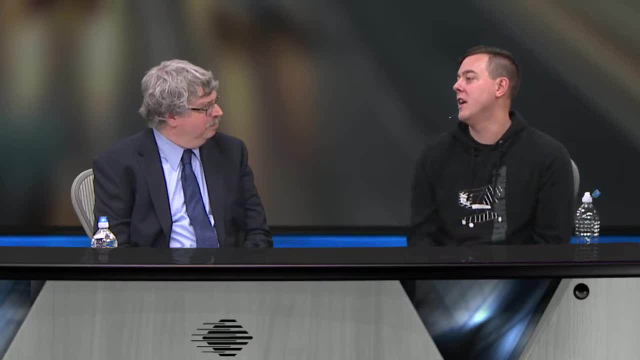 and they would be interpreted to be pushed out to the car's CAN bus. And when we talked about the architecture before, it was that this infotainment system was connected to everything else. So once we had the ability to say, hey, here's a CAN bus. 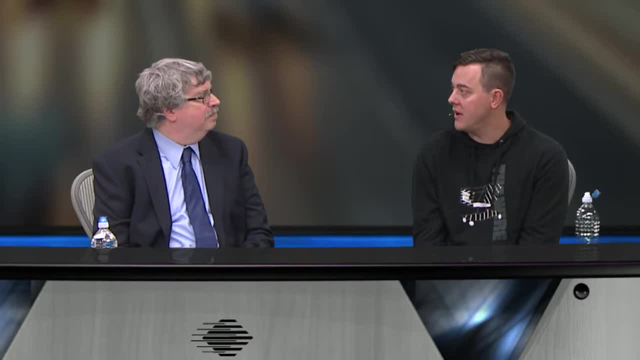 send arbitrary CAN messages. that meant we could actually impersonate any other piece of the vehicle that was using those messages, whether sending or receiving. So at this point you have arbitrary access to send any type of message. Needless to say, we thought it was a bit alarming. But at the time it was limited to Wi-Fi because that's all we knew how to do, which gave the range difference. If I have to drive up next to your car or follow you for some time, that's less of a threat than if I can do anything from say. 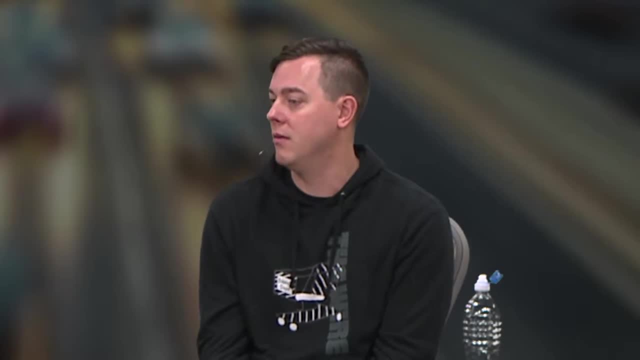 anywhere in the country. We wanted to show that it wasn't a matter of physical proximity but an overall systemic issue. We went back and revisited the code that listened for the certain commands and found out that indeed it listened on cellular. The big issue with that is not only the range, but with the Wi-Fi port And the Wi-Fi port we had to pay, And it was like $35 a month or something, Something that I wouldn't think most normal people would do. 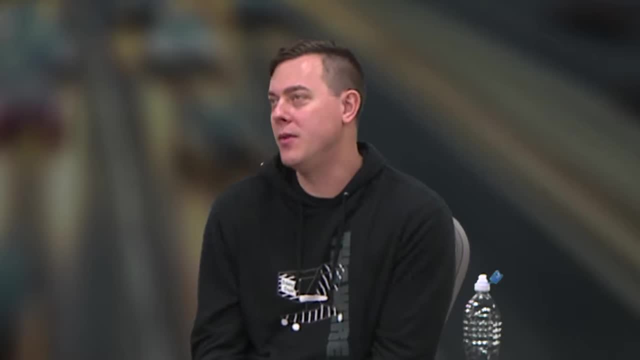 because that's a pretty high expense and you already have your phone, So I wouldn't think many people do that. Maybe they do, maybe they don't. But we wanted it to be a mass scale type of thing And we realized that, indeed, even 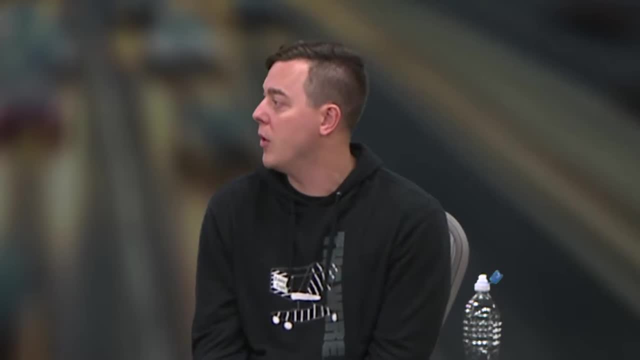 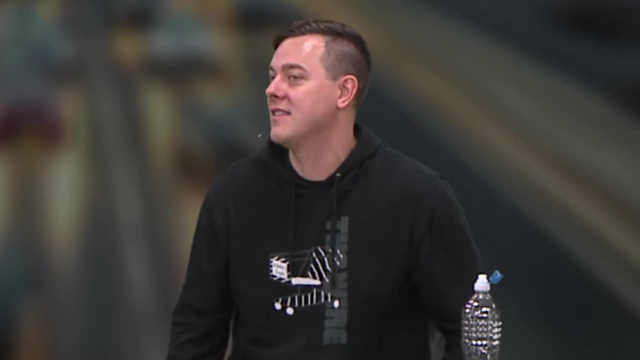 if you didn't have this package, if you had this specific head unit, it came with a cellular modem that you may or may not have known you had, but we didn't know you had. And again, that's another, I guess. 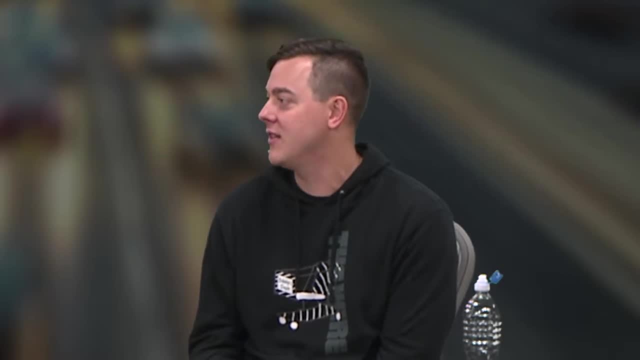 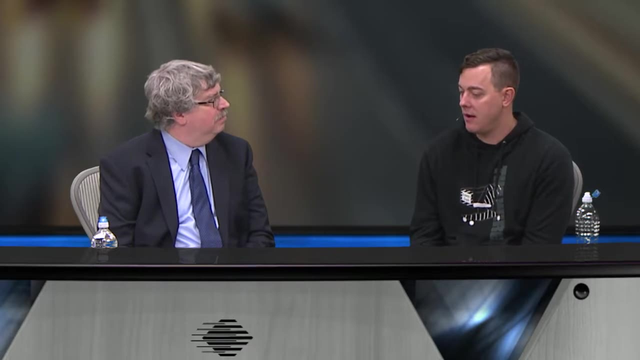 concerning part for a consumer is they don't even understand the technology that's in their car. So is your car constantly connected to the cell towers, regardless whether you know it or not? Yeah, you can communicate with it And it makes sense because they have an app for the car. 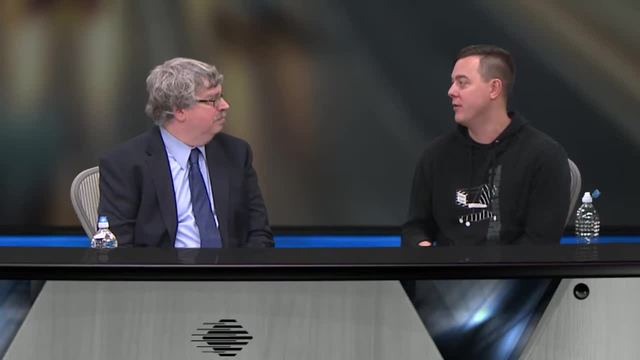 that you can unlock the car and start the car from your cell phone. So you would figure there has to be some level of connectivity, And it was just that We were able to purchase what's referred to as a burner phone Mm-hmm. 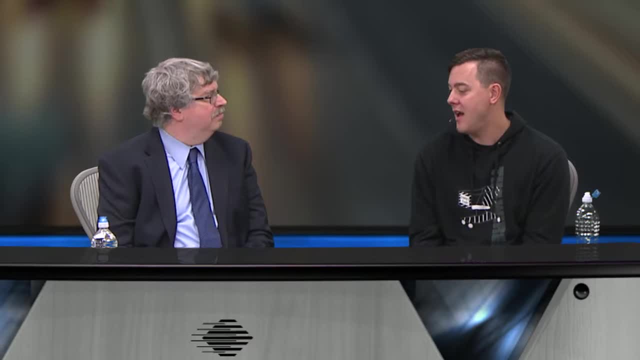 A pay-as-you-go phone from Sprint And we're able then to use that as our entry point into the cellular network that held all these cars, amongst other things, whether it's vending machines or whatever is using the cellular technology. Again, this is concerning because you 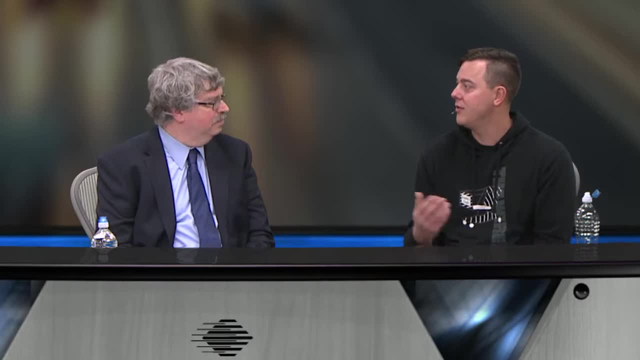 would think that cars would be separated out from, say, your average $20 burner phone that you buy at Walmart. It wasn't So. we were able to get. We were able to get a phone, be it that you couldn't hit the IP addresses from your internet. 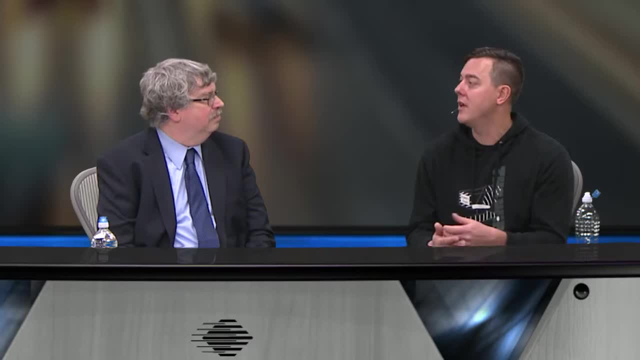 like your cable modem at home, But if you used your phone as the modem then you could actually touch all these things. We proceeded to scan the IP addresses that we knew cars were using For some time. it was really slow because we had a tiny little phone. And we thought there was somewhere between 300,000 and 400,000 vehicles that may be affected out there. We later found out that it was much higher, And they ended up recalling 1.4 million vehicles, So it was a number that was far greater than we ever expected. 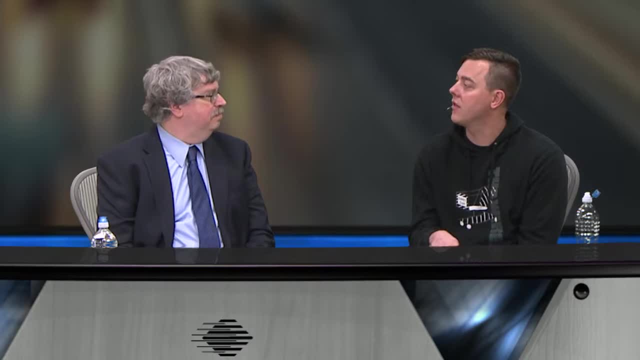 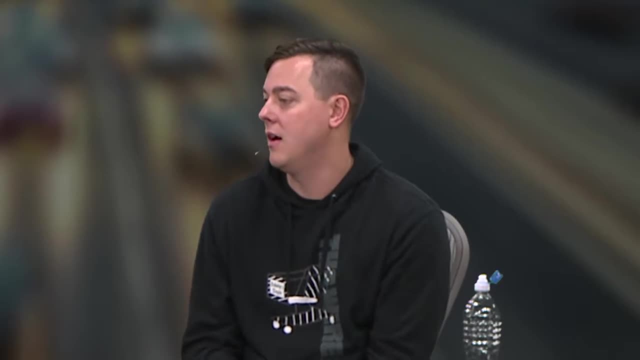 From there, even without doing the process as I previously described, which is reprogramming. there were simple mechanisms for getting the GPS coordinates of a vehicle, getting the VIN number of the vehicle And with those two pieces of information you could tell what make and model the car was. 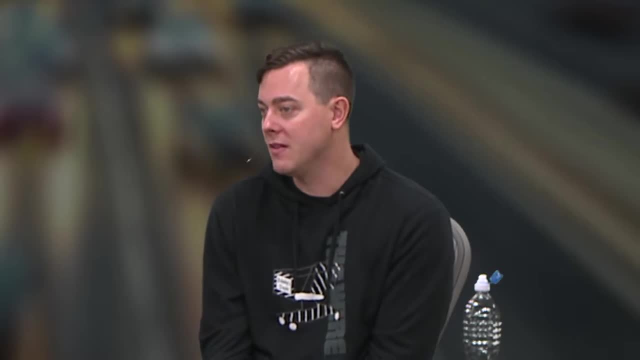 and where it was at any point in time. So less of a physical concern. but a lot of privacy issues stem from being able to say where is this car at And what kind of car is it. So that's essentially how we went about doing this. 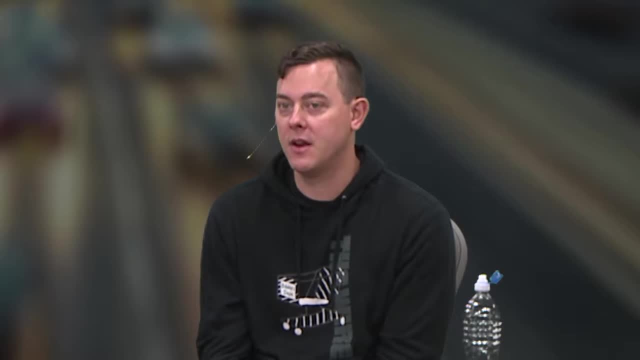 and researching it. The lessons that I like to give out the most is that it wasn't just one party involved. This is an ecosystem, Mm-hmm, Uh-huh. The FCA took basically all the blame because they are a very highly well-respected, highly. 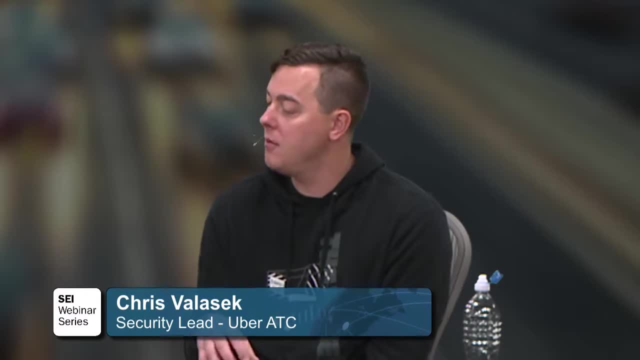 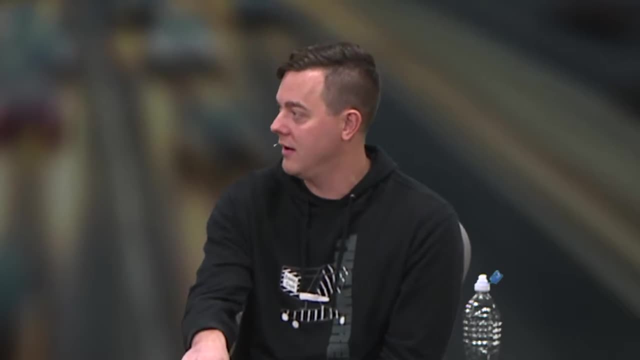 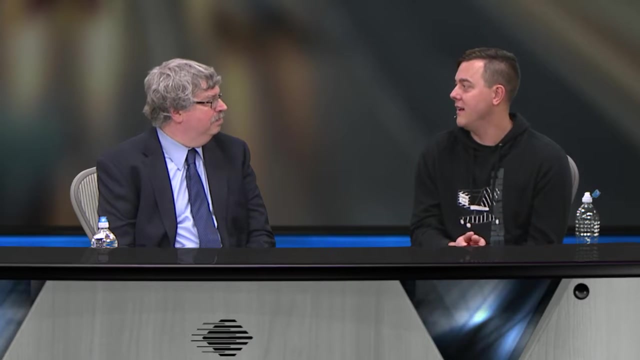 regarded well-respected brand, But at the same time, Harman provided code shipped on an infotainment system that they purchased, And that code was the code that we used to initially get into our vehicle. Secondly, there was Sprint that let just anyone on their network. 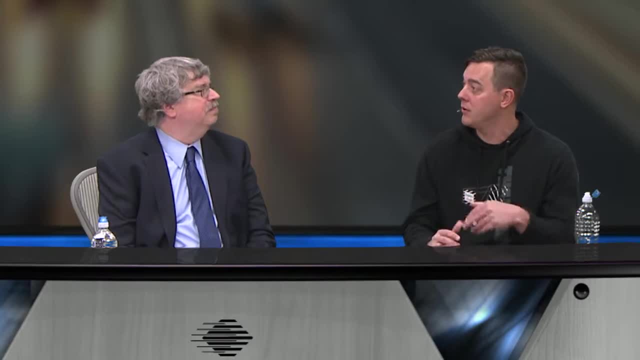 talk to any other device And eventually they blocked that port that we were using to communicate And that had the highest impact right Because now we couldn't do this at scale from our house to anywhere in the country, We'd have to actually get close to the car. 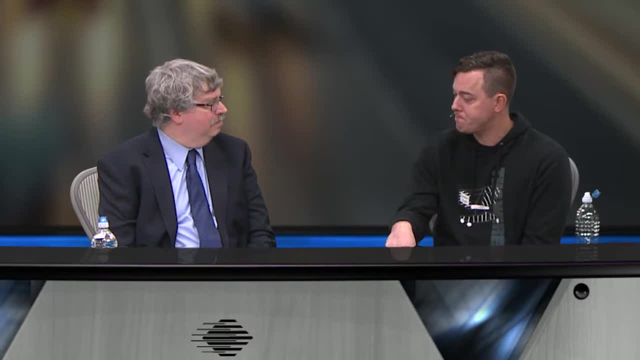 And lastly, you have FCA that's doing these type of updates. They're not checking if code is signed by them. Additionally, the biggest issue with this whole research project from FCA's perspective is the fact that you know we're not. 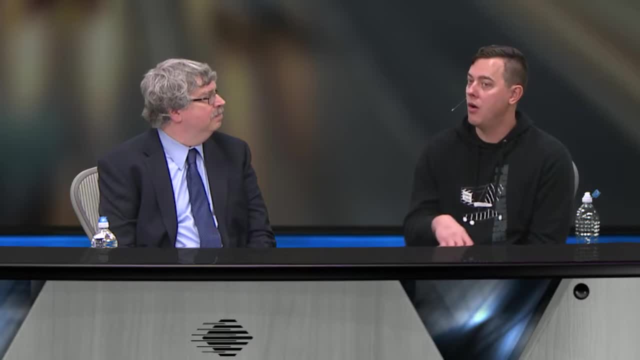 going to be able to update the car And we're going to have to get it back to the factory. And then we're going to have to get the car back to the factory And we're going to have to get the car back to the factory. 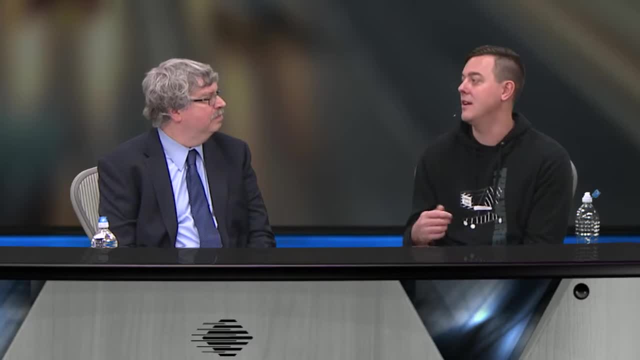 And so the biggest thing that they had in their perspective was they had a machine that could communicate over the airwave, but they didn't have a way to update it, So they had to send out USB sticks and do a full recall. So I think this would have been probably a different story. 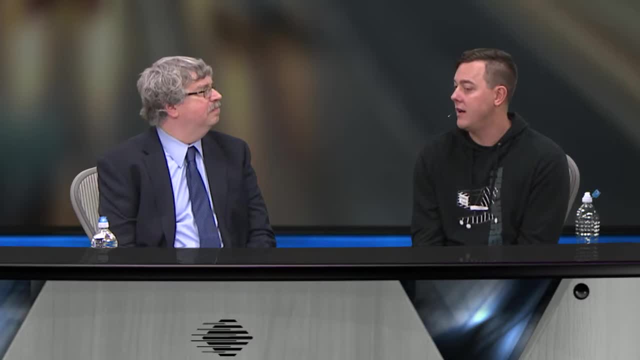 if they were able to say: oh, we have. you know, Chris and Charlie have identified this issue and we can fix it today or tomorrow, right without having to bring their car in. Although wasn't one of your abilities, exploit was the fact. 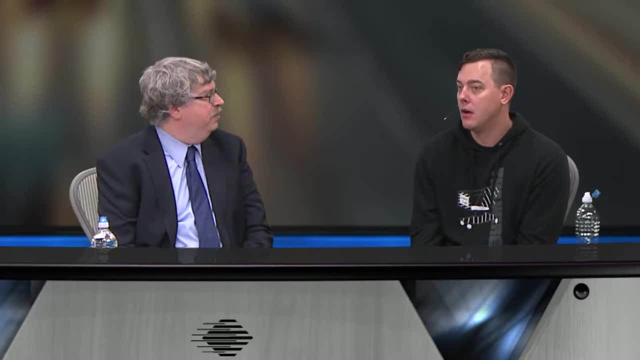 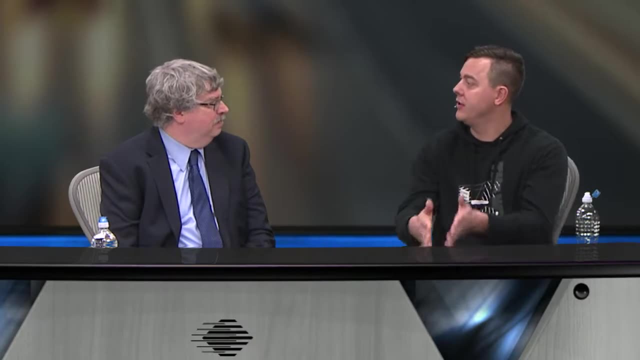 that there was this update capability in those boards that they hadn't put in that additional wire in order to do a firmware update. you wouldn't have been able to get at that. Yeah, but they had no access mechanism to do over-the-air. 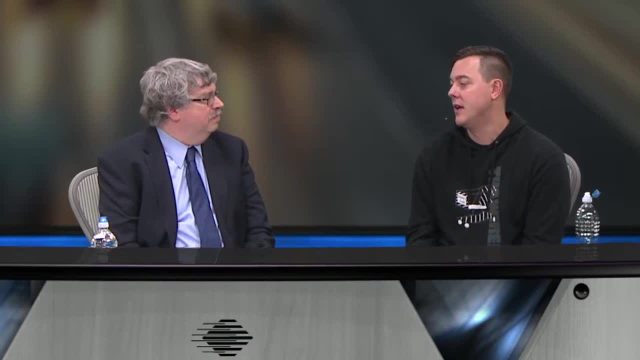 updates is what the biggest, one of the biggest problems was. There's still systemic problems like not code signing that still exist on the cars today, right, but they stop the external effort, Right, and other industries like in aviation. 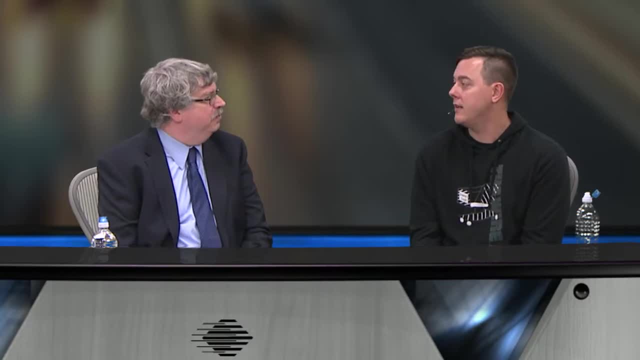 the software that goes into the sensors and engines is signed for exactly that kind of reason. Yes, exactly. You want to verify that the party put in code on here is actually indeed you and it's not an altered form of what you're putting on there, which is exactly what we did. 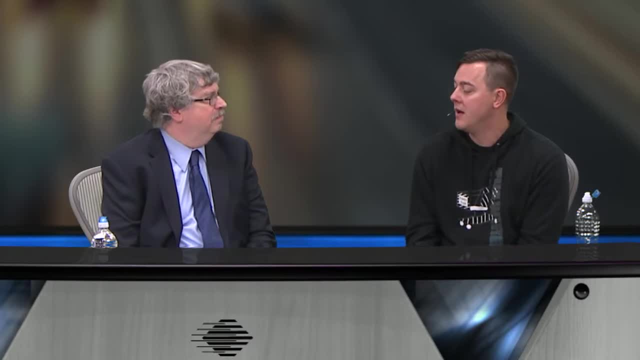 We altered their code slightly to do what we wanted. Yeah, so you know, code signing for these type of applications is highly critical, even for your phone. I think Apple learned that pretty quickly- is signing all their code and not only signing their code. 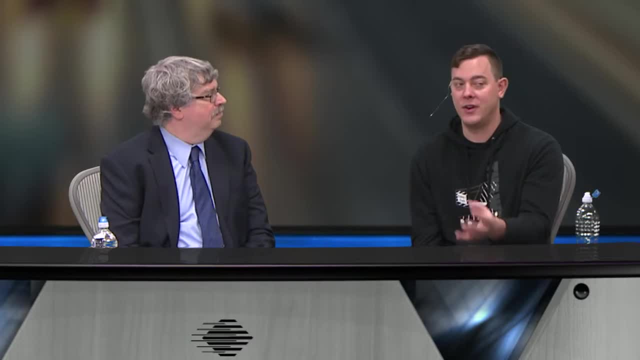 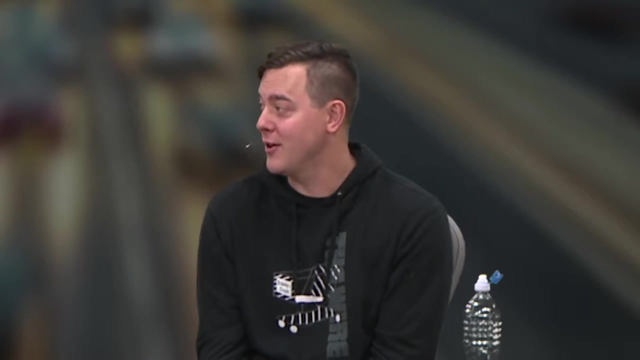 they're signing their memory regions right. You don't want people putting their own data on these devices for safety reasons And, you know, many times, reliability reasons. Now it does bring up a kind of conundrum for people that like to tinker with their things. 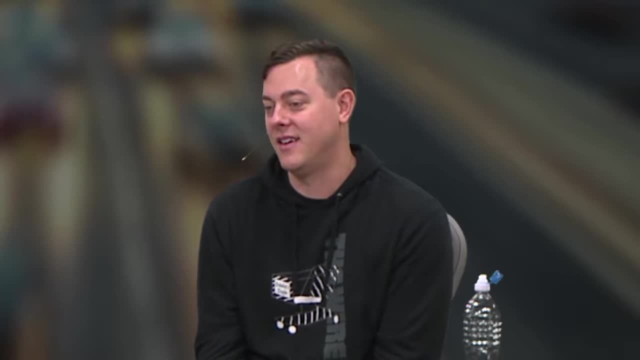 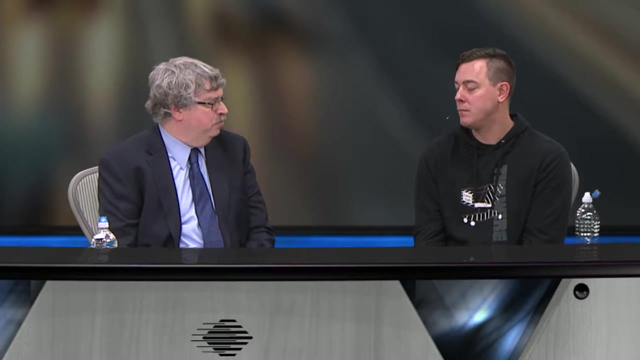 as someone who enjoys that. but you know, I think many times, especially for this firmware level access, that having verified and cryptographically verified code on them is the way to go. You mentioned that this was sort of step two in the study. 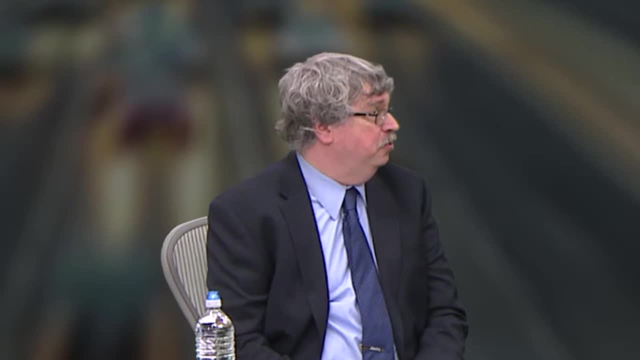 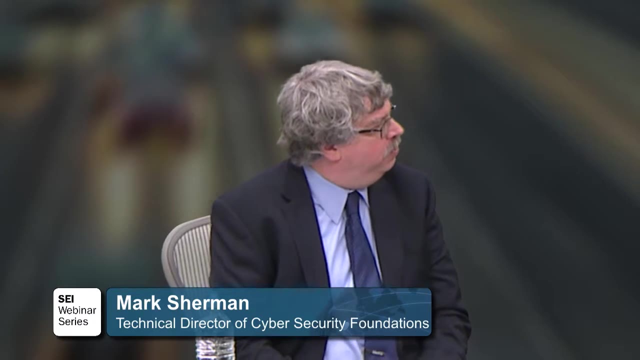 step one was doing a survey of the various architectures, and then you picked the Jeep as one that looked most promising for vulnerabilities. What would you say were some of the better architectures that you saw? Yeah, I mean, unfortunately we couldn't some. 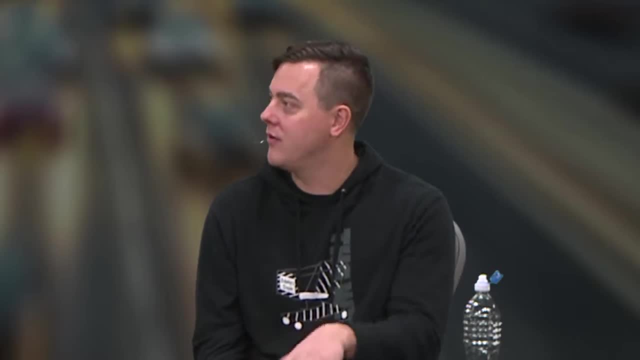 I-O-Active at the time bought us the Jeep And apparently they wouldn't buy us one of every car on the planet, unfortunately, even though we wanted it that way. But yeah, the architectures that we initially shied away from had separation between the two. 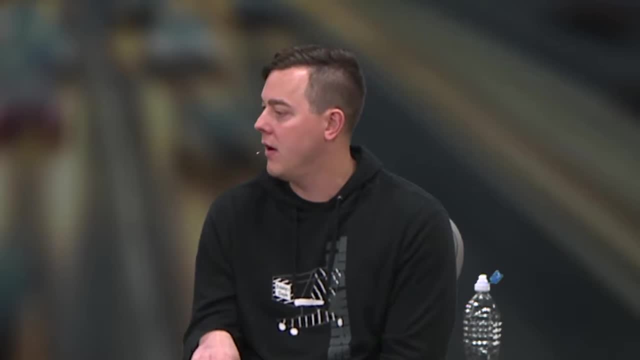 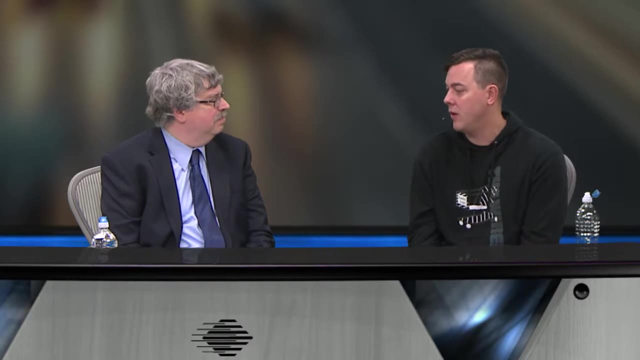 There was a separation between some kind of gateway unit, between things that communicate with the outside world and things like engine controllers. There were even more sophisticated ones that you know: steering was on a different portion that was separated by some kind of gateway than braking. 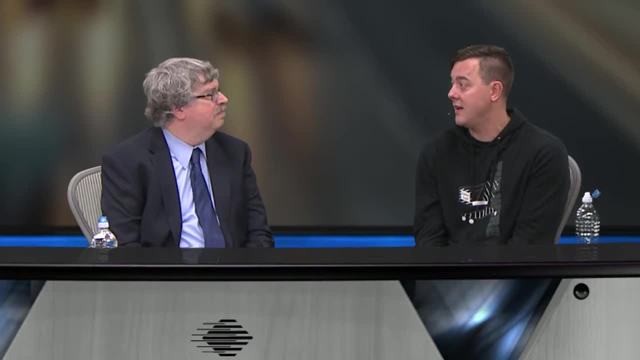 and all that stuff, Not to say that's perfect and it was worked as designed, but needless to say, we didn't want to try the hardest thing first, right, Yeah, so the just like your, you know computer networks that you have in your offices. 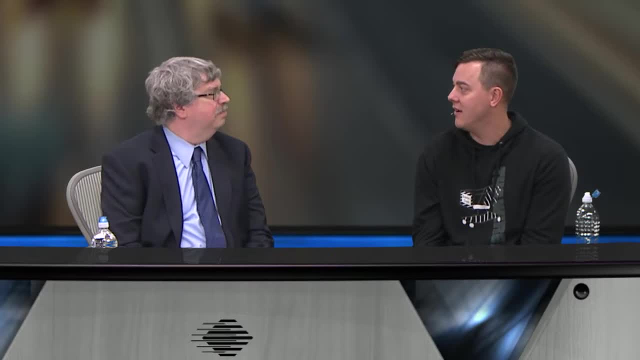 and corporations. right, You have some level of separation. People from finance shouldn't be accessing code repositories on different parts of the network. Database servers that are holding highly critical information shouldn't be worldly accessible from the outside. So we're taking the same kind of concepts. 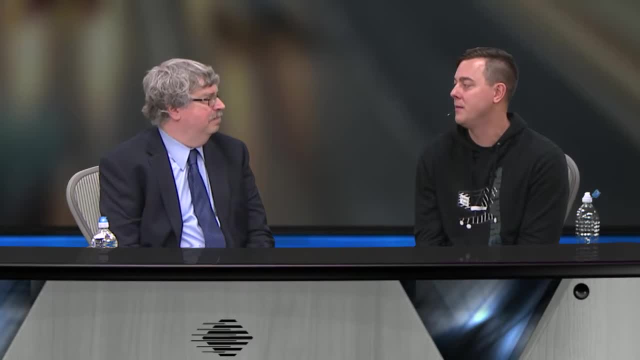 because they really do apply to these machines as well. One of the last, I guess, portions that I do like to mention as well, probably just to save more face than anything. I think a lot of people saw the video right And it did prove our point that we wanted this to be real. 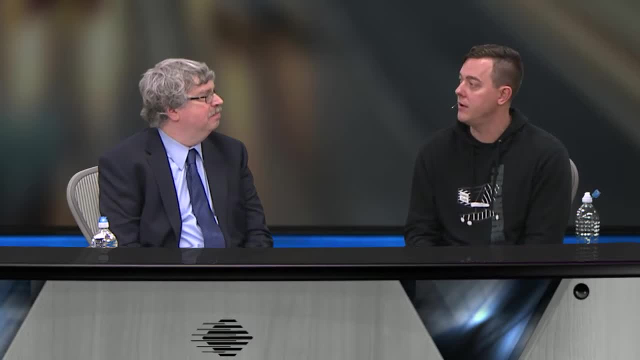 And I don't think it would have resonated with as many people if it wasn't real, if we were doing it elsewhere. But we worked with FCA for almost nine months prior to this, So this wasn't us just dumping something on the internet one day. 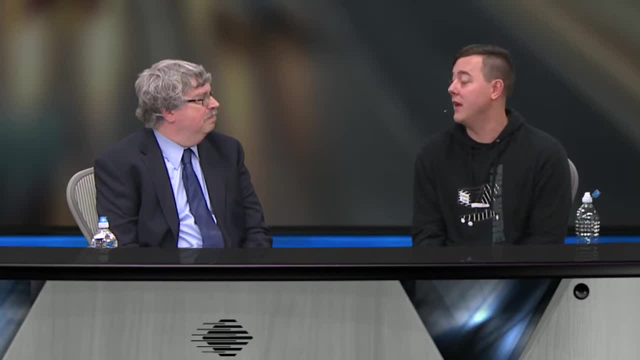 I mean, we were working with them, we explained to them what we were doing and we told them that we were doing the Wired piece and everything like that. So I do encourage research, research, research. I encourage researchers and everyone alike. 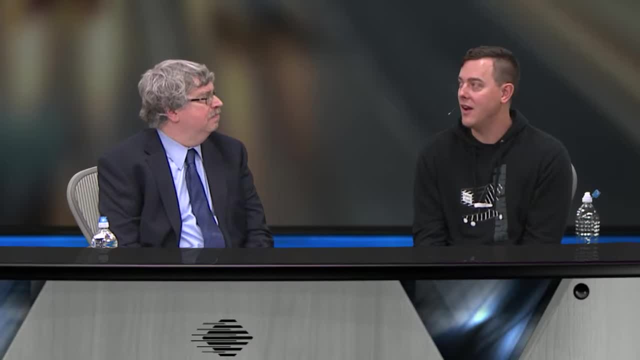 to coordinate with these people. You have to remember that not everyone comes out of the womb being a security expert, as you obviously know. It takes time and it really takes buy-in. For example, I was prior to doing automotive research. 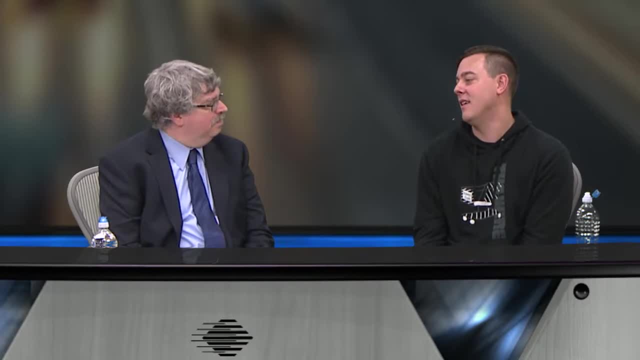 I was a Windows hacker and they really didn't get serious about security until Bill Gates' company-wide memo that said: hey, we really need to take this seriously if we're going to be in this market And I think some of the first big battles. 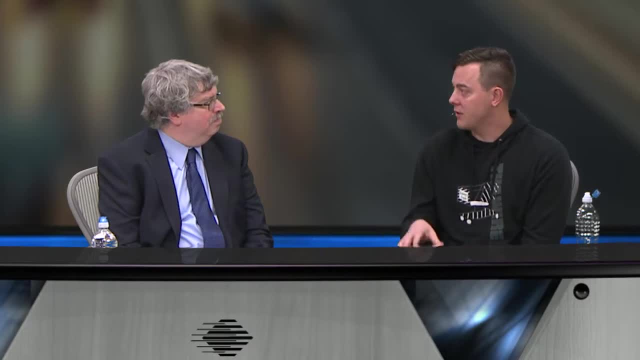 that will be fought on these fronts, specifically with cyber-physical systems, is buy-in from the top down, where this is a priority and important and it needs to be built in as they go along. But does the Wired author still talk to you? 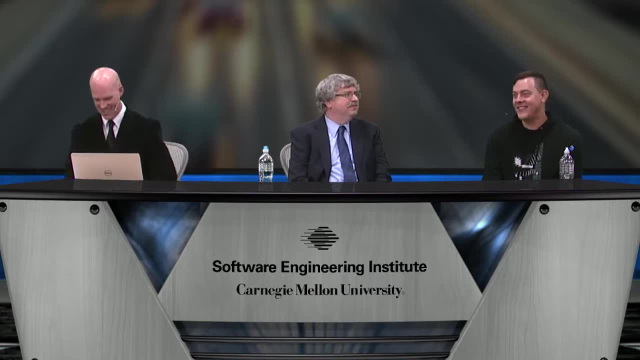 after being in the car. Yeah, Greenberg still talks to us. He's a really nice guy. He asks if we're doing anything new. He said he'd be the first to call us. He'd be the first to call. I like Andy a lot. 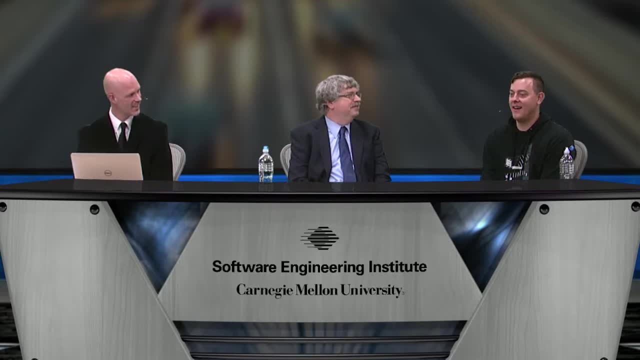 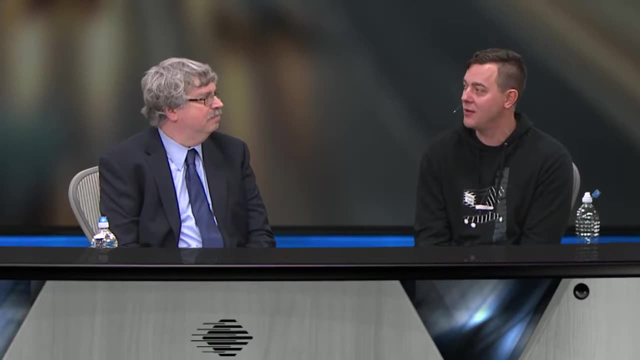 He's a great journalist. Is FCA still talking with you? We haven't talked to them much since the events that unfolded. yeah, But they were and I'll commend them on this. they were really cool about it. There was never any legal threatening. 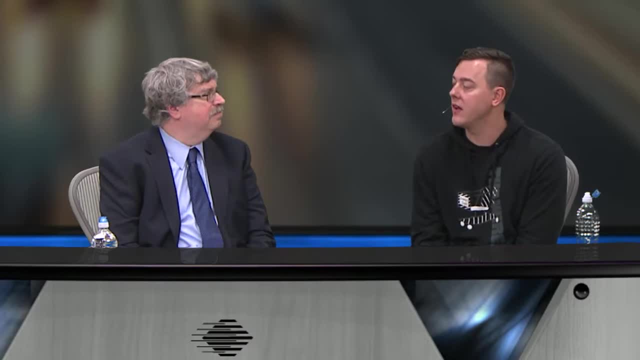 They asked us to view a few things. We thought it would hurt the integrity of the research and they didn't really have problems with them. So for all intents and purposes- I'm sure there's- they may not like us, but they were very respectful. 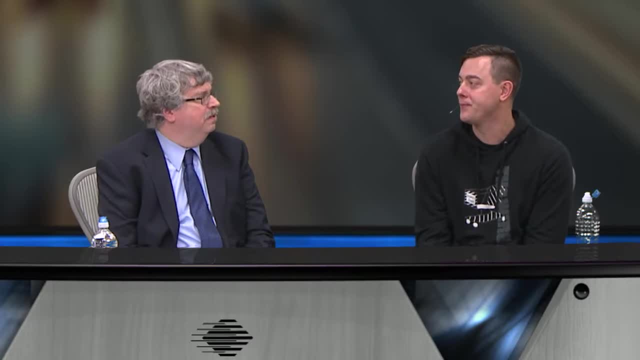 the whole time and I think we were on the opposite side. You mentioned that you did a fair amount of reverse engineering, basically looking at blobs to figure out what they meant. Who, would you say, has access to that information just as part of their normal job? 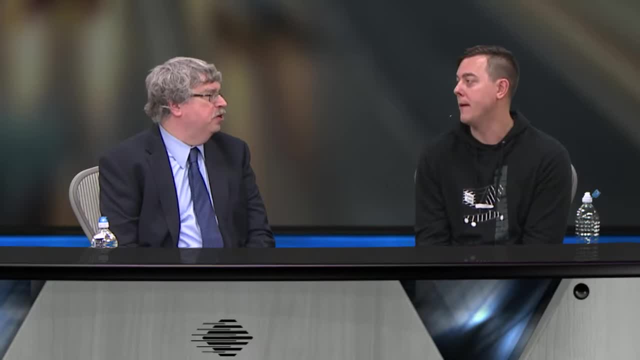 What pieces of information You're talking, like the firmware code. The firmware code or the communication message formats or the various other things. So I mean those are probably internal to the company. As for the firmware, if you know the microprocessor, 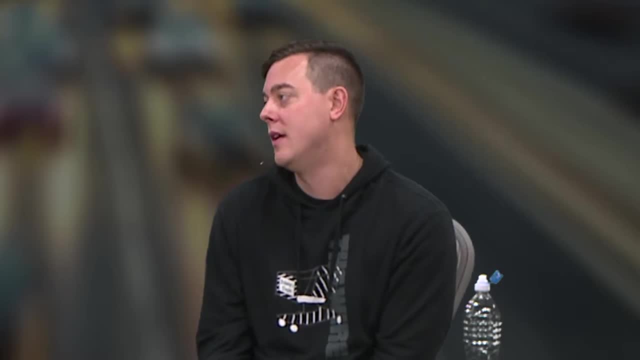 you can open a thing like IDA Pro, which is a disassembly tool. That's what we did and spent a lot of time looking at that. As for the messages the car sent, those are internal to the company and not published. 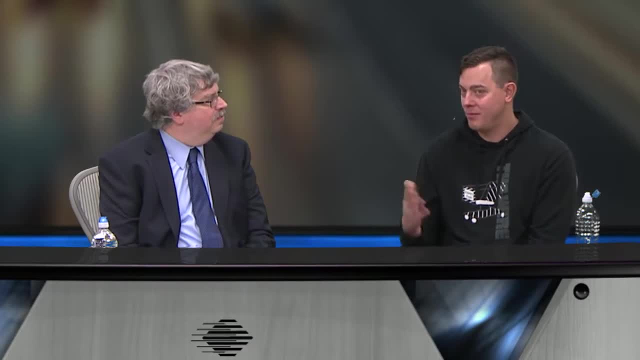 So that was us just reverse engineering A lot of times making the car park itself, and we wrote our own software to look at the network communications and say, oh, this looks like these bytes are changing as the wheel's turning, or this happens. 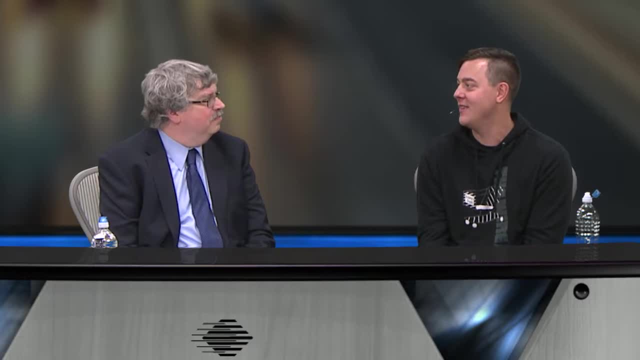 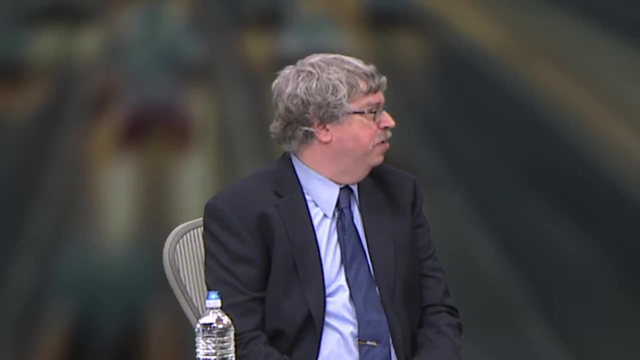 when I press the brakes. So we would do that. So that's what we did. Spent a lot of time out in the car. So much of the systems for things like cars have contractors. Harman Kardon is just one of them. 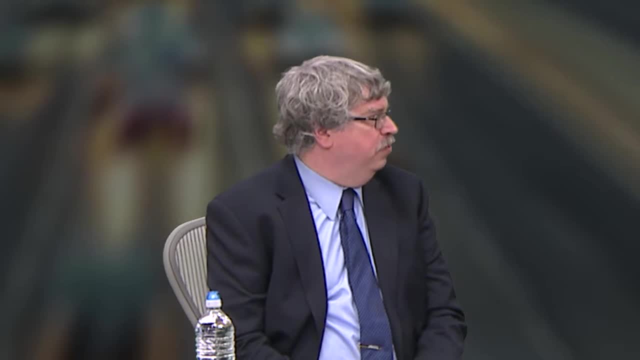 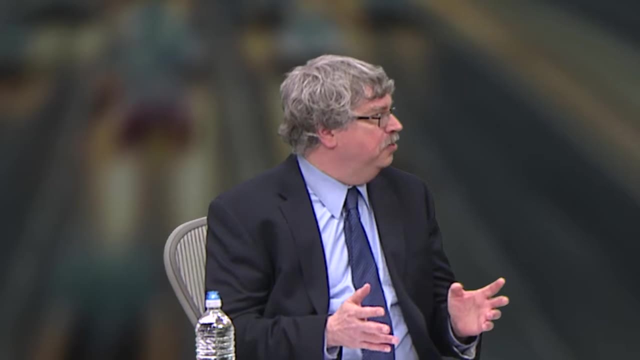 In order for all of these various companies to do their jobs. if you have all of these units throughout the car, dozens and dozens of units, you'll have to talk to each other. You'll have to not step on each other. How many people would you sort of sting a finger in the air? 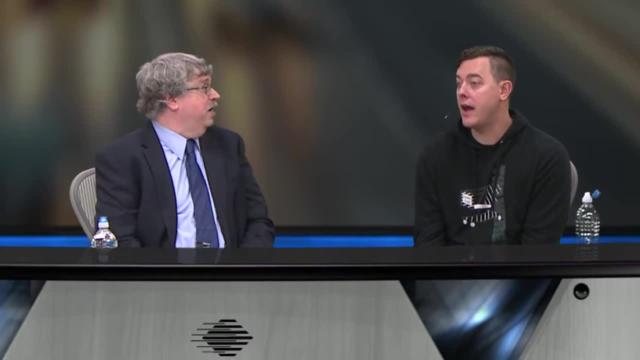 would have to know these various things in order to make sure that it all works together. I don't know Lots of people, though I would assume a lot of groups. I'm only a hacker, so I only know how to break it. 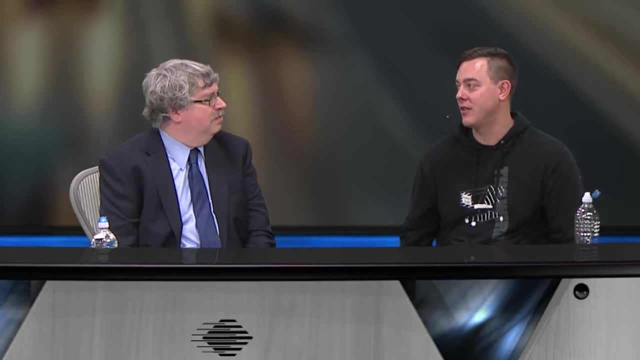 But I'm sure building it is much more complicated. So there's a lot of people involved in all these steps. So might a disgruntled employee in any one of them be able to do what you did a lot faster? I don't think so. 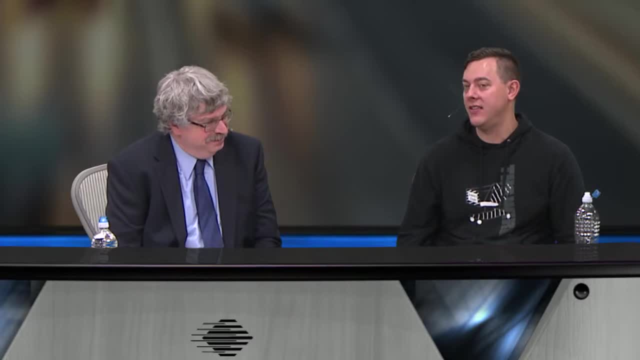 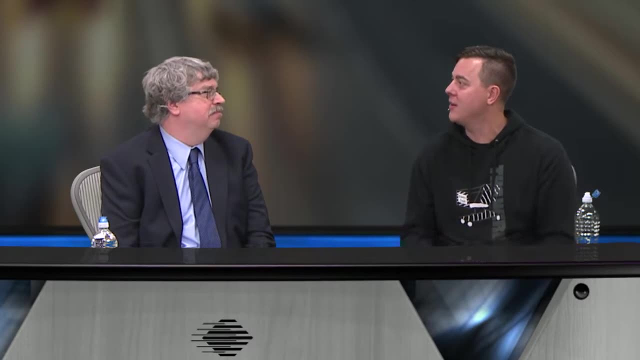 We're too good. No, I don't know. Yeah, they would definitely have an advantage to having information that took us weeks to derive, where they would have an actual document explaining what was happening. for sure We originally, when we first started- 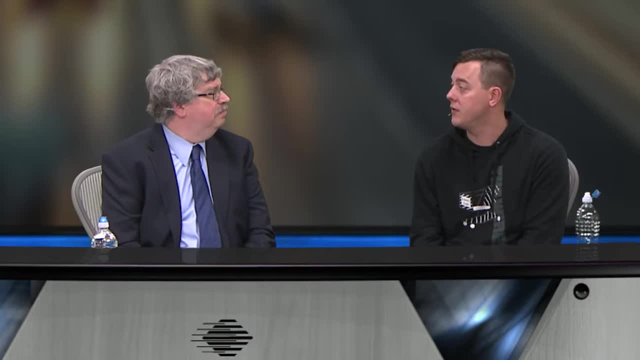 doing automobile research back in 2013,, were trying to figure out what the messages were like And we thought we could just buy them. Apparently, you can, but you have to sign some paper And it costs an exorbitant sum of money. 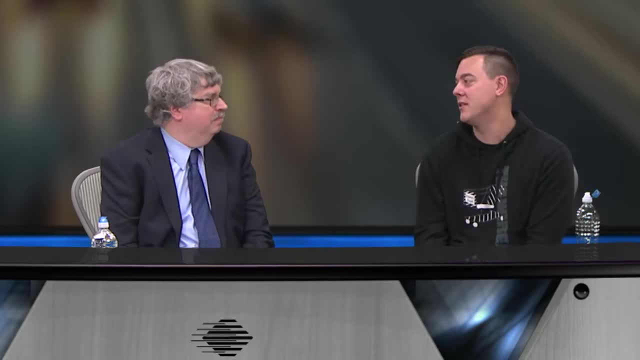 to get those type of databases that have the messages. So we just figured we'd figure it out ourselves. save ourselves a lot of money, So a well-funded adversary might be Yeah, right now for a lot of these well-funded is a prerequisite to the whole thing. 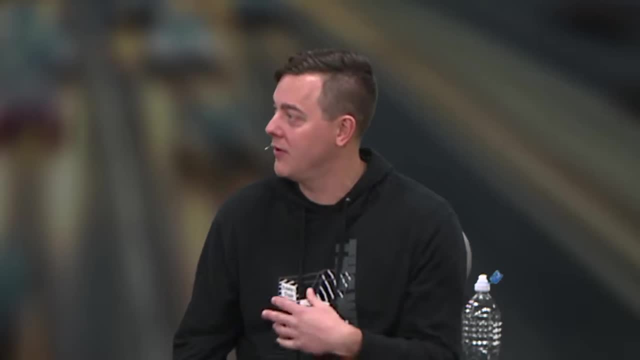 Now we had the car right Because we weren't going to test against strangers, We only were testing against our car. Additionally, to figure out those messages: if you're not going to buy them, you want to purchase a vehicle. 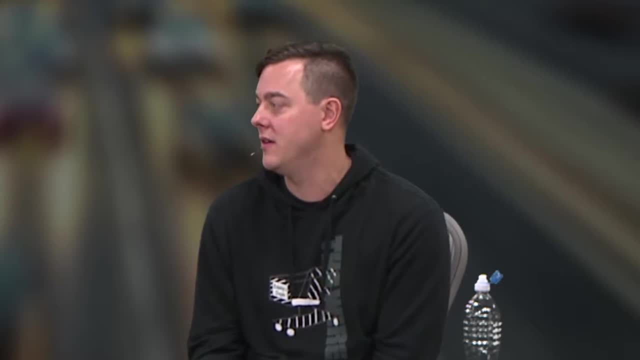 So the barrier of entry to this type of research is pretty high right now, because even that Jeep with the technology packages was somewhere in the realm of $30,000 plus $1,000.. So this isn't a weekend project that most people pick up at home. 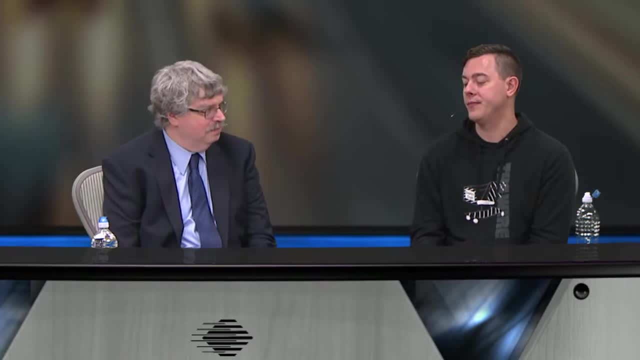 You actually have to have some funding to get involved in it, Mm-hmm, Fantastic. Well, do you have any recommendations at a high level on how you would go about securing these types of systems? Well, in just listening to your discussion, 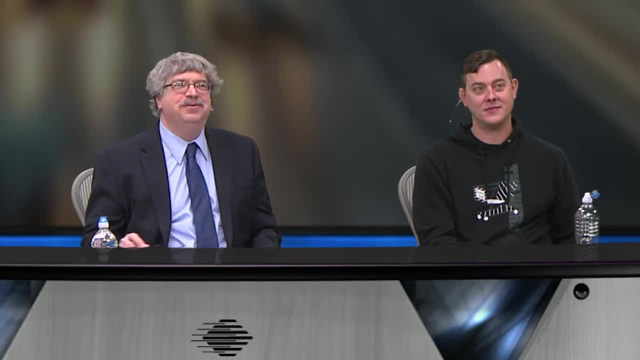 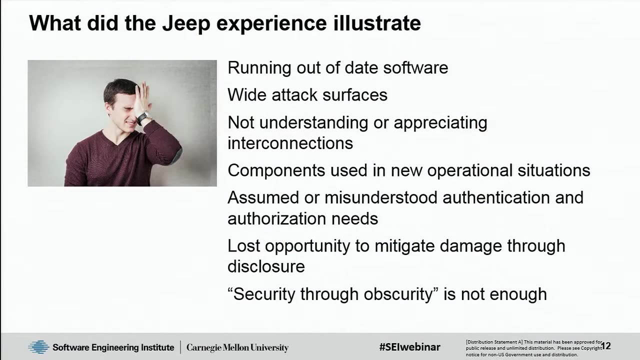 and I have to admit I've heard you give this a couple of times already. There is a variety of things that I think you saw, illustrated by your experience with the Jeep. A lot of the software and some of the components you were talking about was out of date. 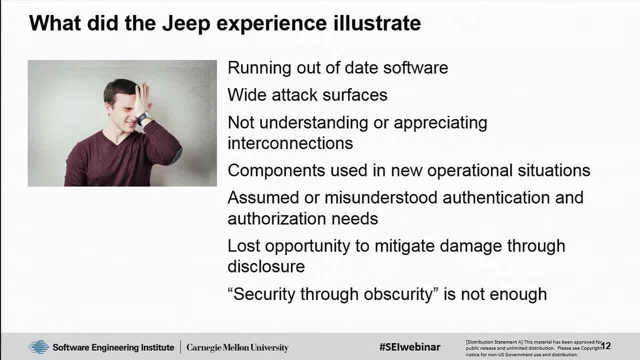 And there were known issues with those software and sometimes even fixes for those software that were simply not applied. We already talked about that. there's a wide attack surface that by design they created lots of ways in which may have been partitionable that we saw in other kinds of situations. 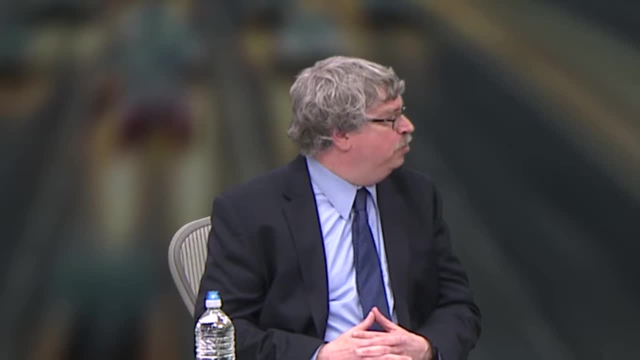 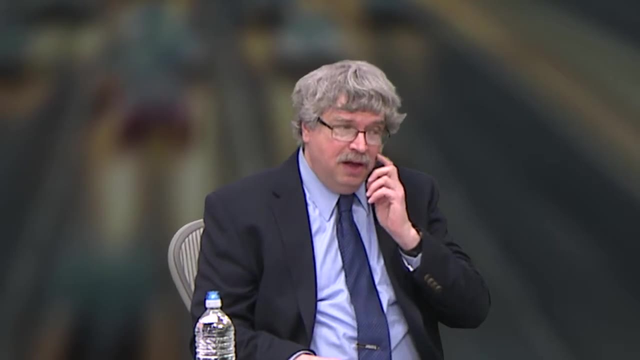 Sort of a lack of either understanding or appreciating all the interconnections between the system. The fact that the serial line was placed between these two boards meant it really wasn't air gapped, even though it may have been described as an air gap. 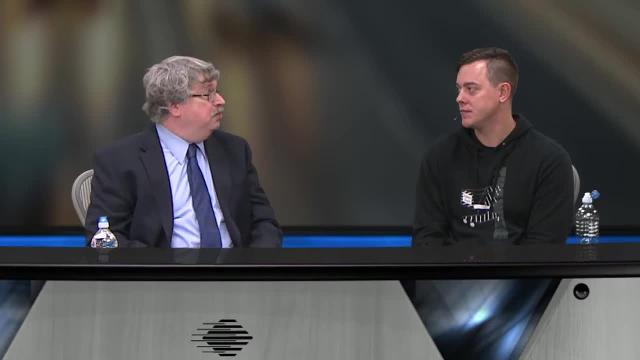 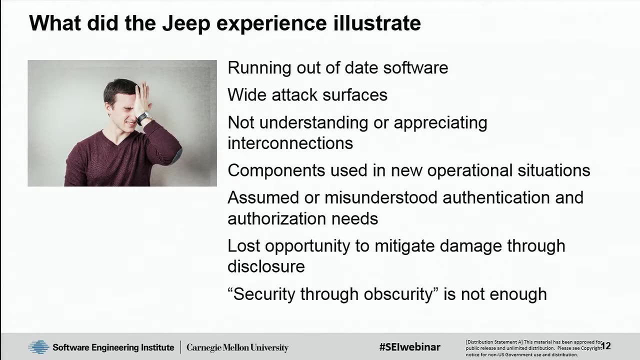 Something that you also mentioned, which we actually have seen in the research literature as well, is that when you use a software component in a new operational situation, you almost always find a vulnerability Here. as you said, the braking system was never intended to be connected to a front end. that 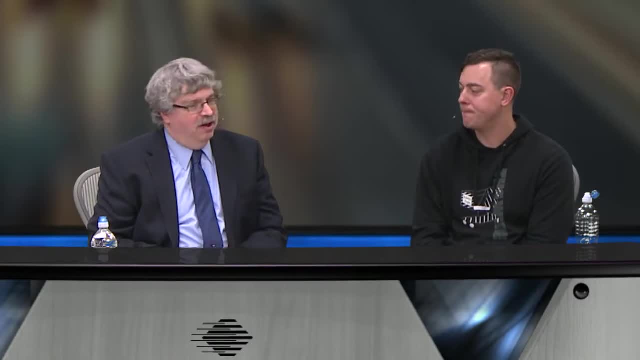 connected to the web. When it did all of a sudden, the path was there. The studies have shown that In general, when you introduce a new piece of software, that the first defects you find are in functions in the new code. 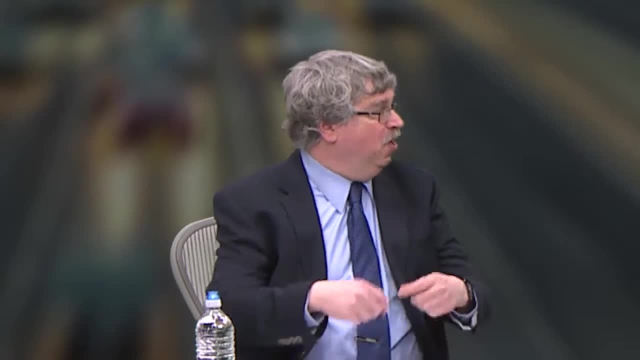 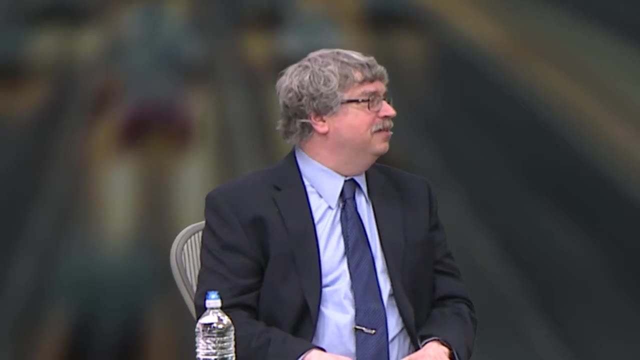 but the first security problems you find are problems in the old code. that's now put in a new kind of environment And this just showed that in many different ways It gives the old code new context. Yes, unexpected context that whoever was building it. 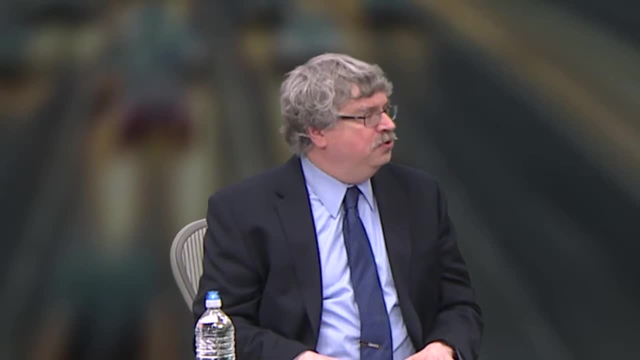 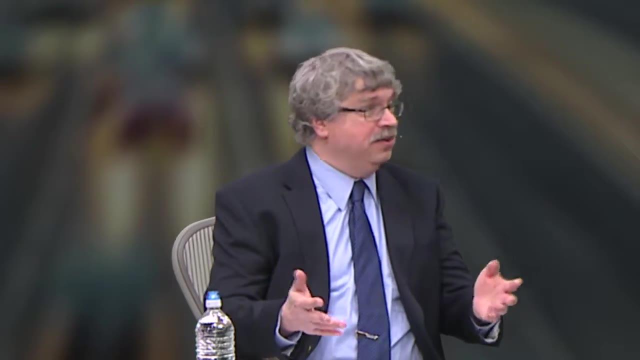 never thought that, which again led to there was sort of an assumed or misunderstood need for authentication and authorization. Yes, There's no need for signage. We're just finding who's going to do it. only the mechanic. We trust the mechanics. 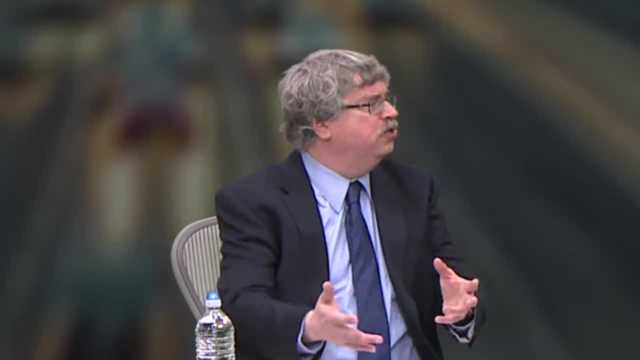 The CAN bus never has to look at the messages, never has to verify who's coming in with the message, because it's all written internally. We know no one from the outside is ever going to do that. Well, no one from the outside now did. 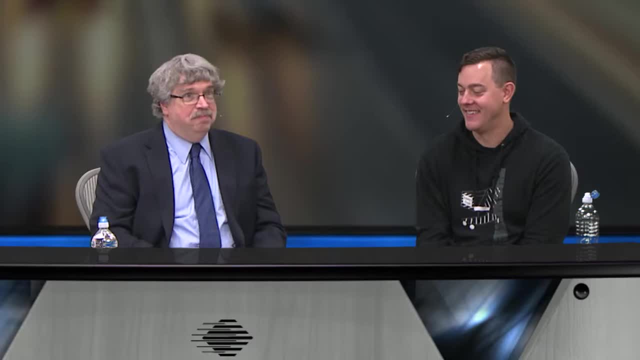 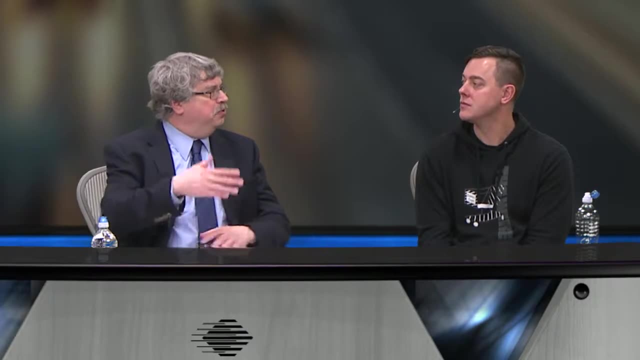 And so all those assumptions have now been changed. We also saw what I would say was sort of a lost opportunity to mitigate the damage. As you said, you were in constant contact with FCA throughout this process, But it appears from the outside, because I'm not- 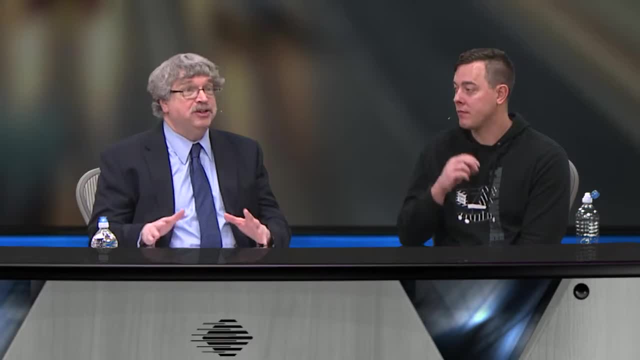 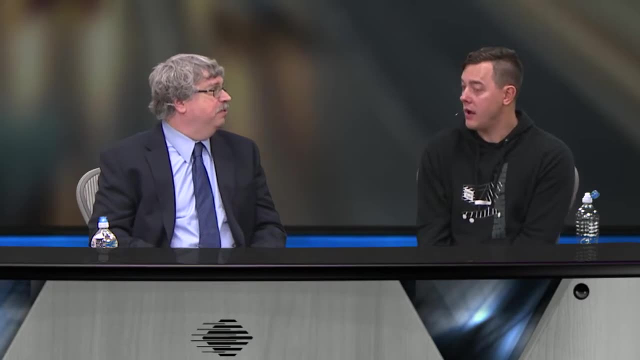 with them either. so I don't know. But from the outside it appears that action was only taken after this went public. So after the article came out, then Sprint did something, Then they started to do something. Yeah, we didn't release anything until there. 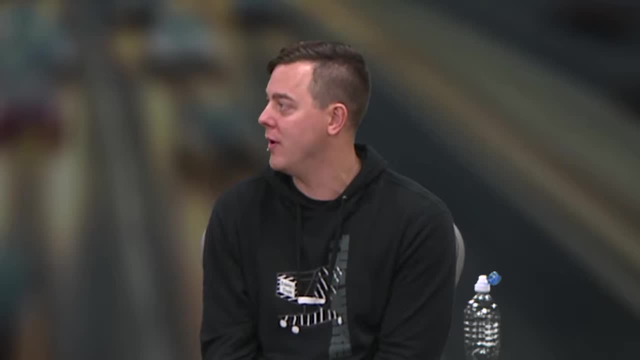 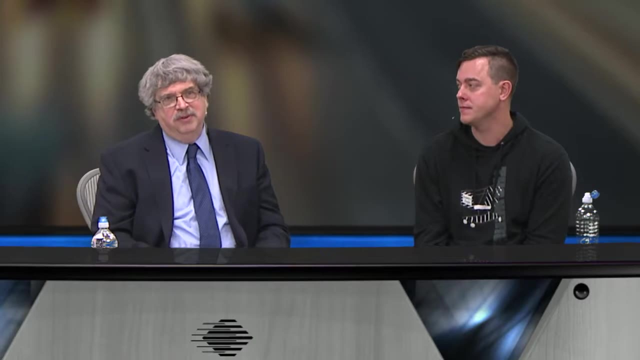 was a patch available. But after the Wired article and our kind of media tour thereafter is when Sprint took action and it really accelerated. So that was also something we might learn going forward. And I sort of summarize it: I think that's the last comment which 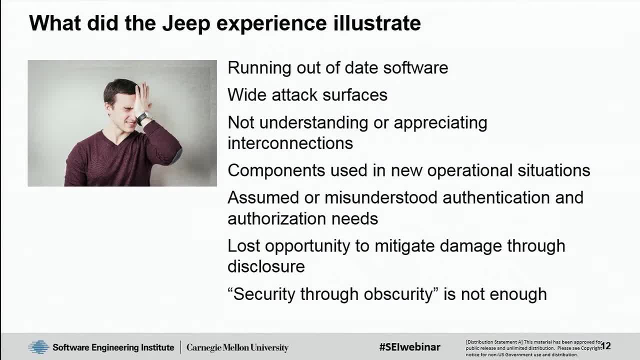 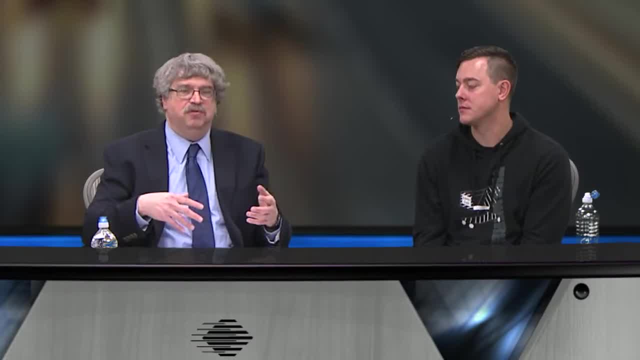 is that security through obscurity is not really the answer. There seems to be a belief, especially by people who are focusing on feature function, that we don't have to worry about this because this is a very complex system. It's very hard to use. 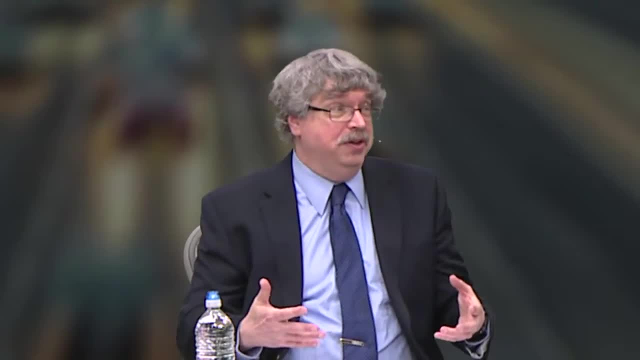 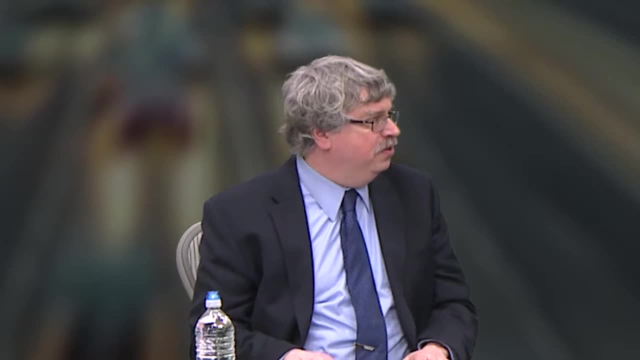 You need to know a lot of things. It's just not going to be worth anyone's while in order to go ahead and do this. Well, there's just many examples of which is being the last one, and where you just can't rely on the complexity of what the environment is in order. 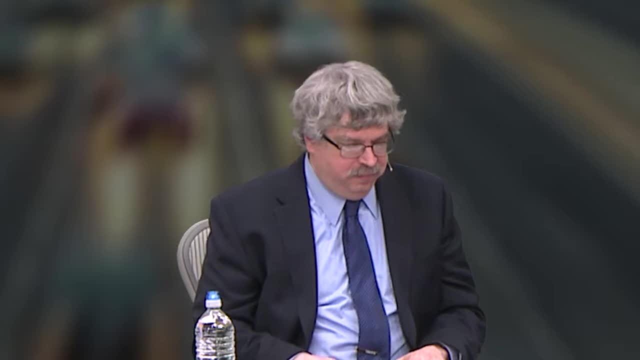 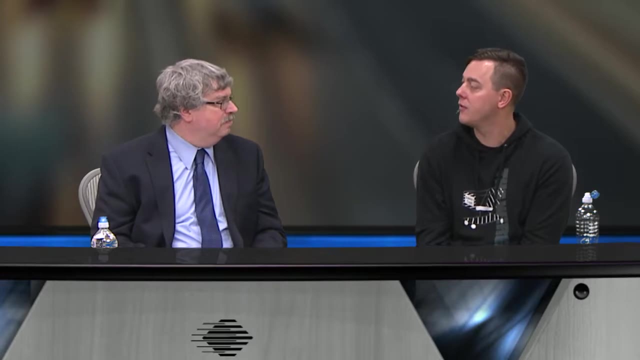 to actually solve your security problem Exactly. We weren't even the first people to do this, remotely, if you'll believe that The researchers from the University of Washington and University of California, San Diego did this on a GM vehicle back in 2011,- kind of four years prior. 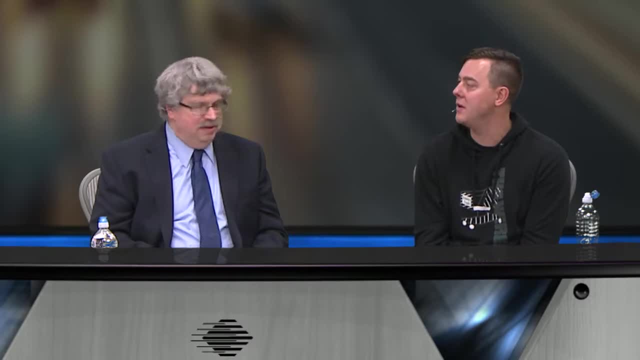 So even if there was the thought process of this may be impossible because it's super hard- that should have been shattered prior to our work. Right, and there have been, I think, several efforts that have done it through the onboard diagnostic port as well. 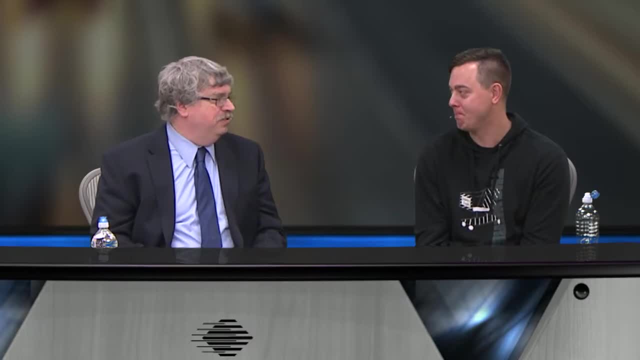 Absolutely So. again, lots of ways in, and any one of them gives you access. The argument on that one, however, is if you can get physically inside the car to begin with. well, I think all bets are off. I can just take the car away. 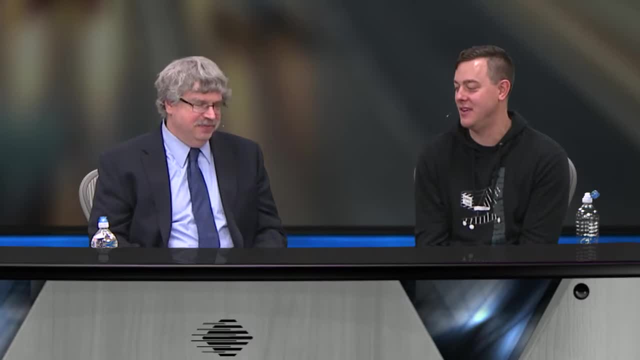 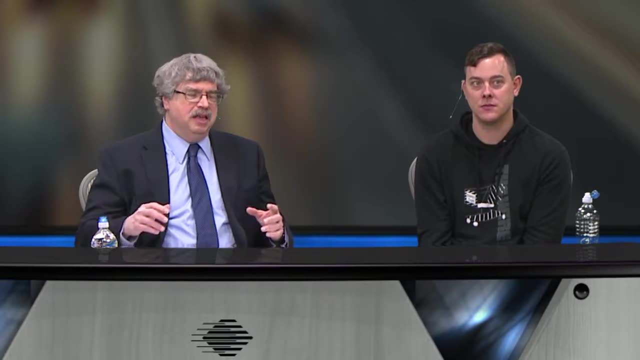 Yeah, you can go traditional kinetic attack if you have physical access, It might be easier, Right, But the reason why we're here and why we're trying to focus on this is that if you see these kinds of things early, it's a whole lot cheaper. 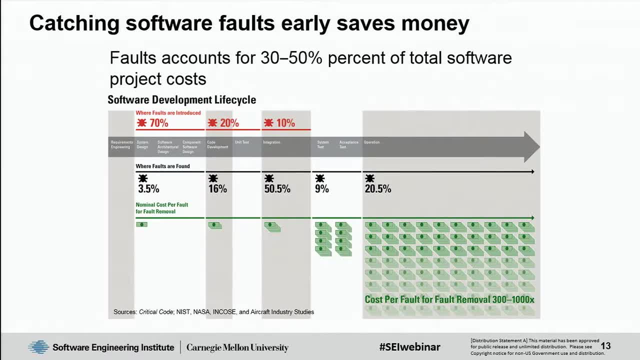 to fix that. just in general sense, if it costs you $1 to fix something up front, it can cost you up to $1,000. And that's ignoring any other kinds of implications. So, like in the case of Jeep they. 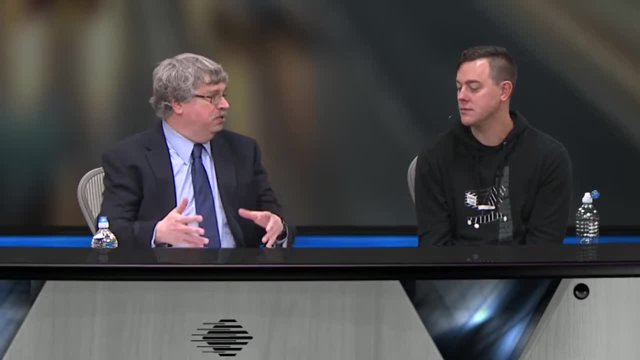 spent hundreds of millions of dollars in a quarter that they got hit once this disclosure came out- Although not really a security related event, but the Toyota event, which is a software related event. depending on who you're counting, it was somewhere between $1 and $4 billion of impact. 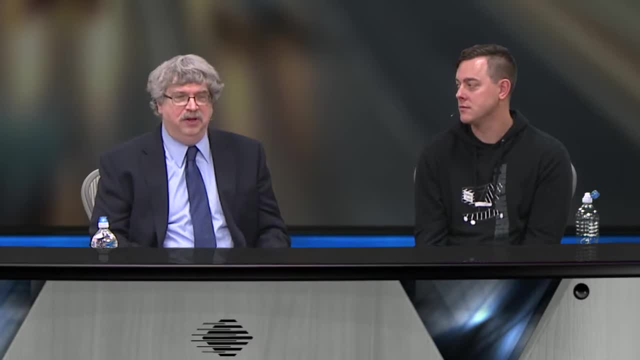 Yes, it might take another developer. Yes, it might take a couple of week impact to the schedule. Maybe take a little bit more memory if you want to do some of these things, But the flip side is the cost of not doing it. 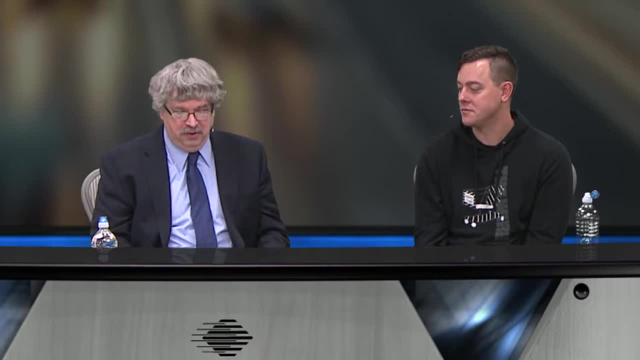 and coming up with it later- is just staggeringly enormous, And it seems to be increasing, And so what we're going to do for the rest of the seminar, the rest of the webinar, is really focus about how one addresses these in the security life. 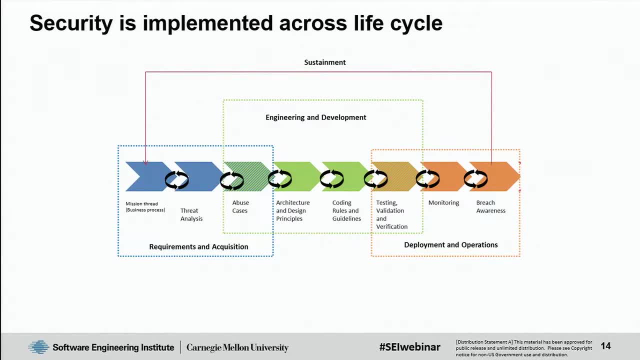 cycle in the software life cycle, with the key message being: we know a lot of things that can be fixed right now, That, as you mentioned, even in the Jeep, the example that you gave, there were lots of things that could have been done better. 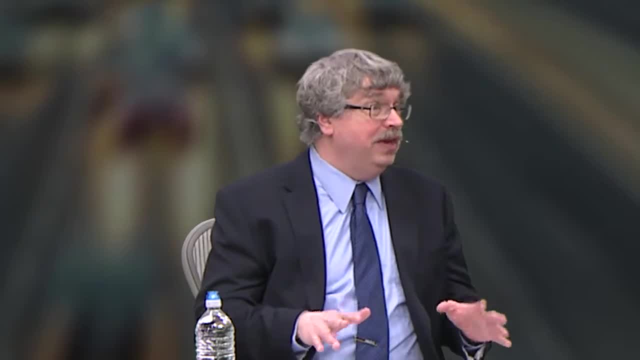 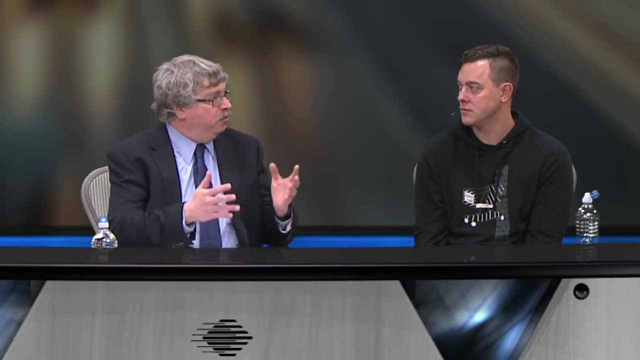 that would have made this much, much harder, Not impossible, but we can get a lot better than we are right now, And to do that we're going to take a look at both the beginning requirements phase, understanding the threats, understanding the threat models, just like we did here. 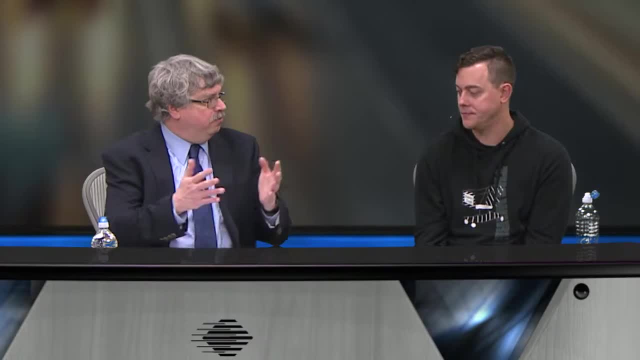 with the attack surfaces, the architecture and design phase, looking at how to separate things, how you want to actually encode, and then going into operations. How do you make sure what you have is working And when something goes wrong, what to do about it? 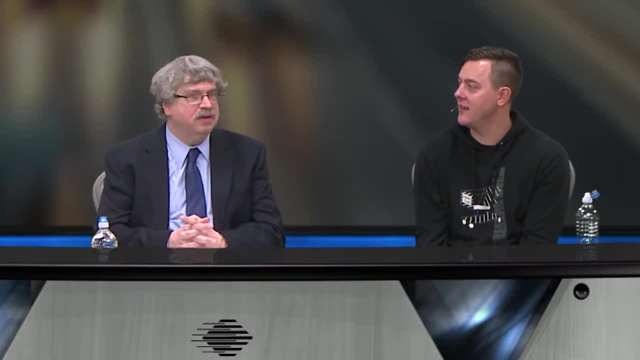 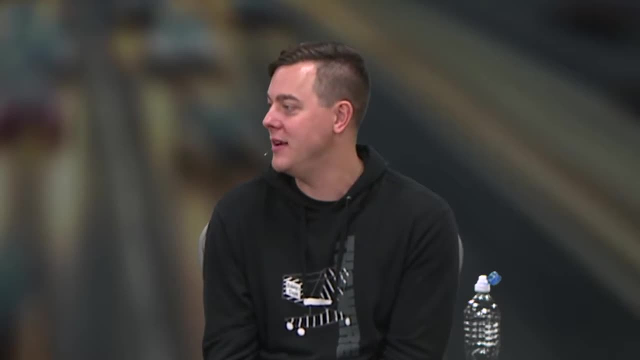 rather than saying oops. I think that's one of the biggest issues. that gets overlooked is assuming that if you can make security perfect, it's not something you can make perfect and you want to be able to remediate when there is an event. 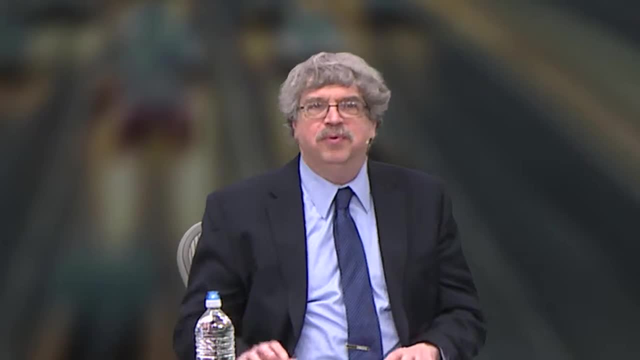 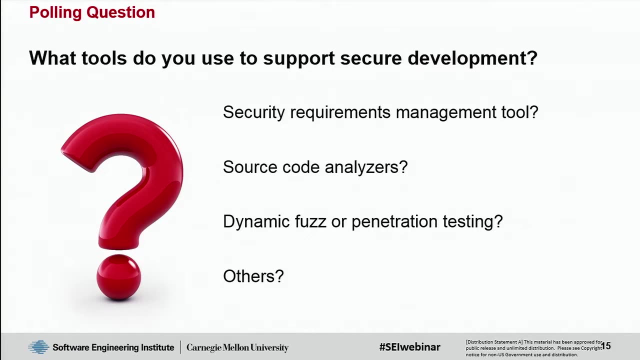 Yep, Thanks. So with that, let's come to our first question. So, like I mentioned in the intro, folks, we'll ask a number of polling questions throughout each talk just to get an idea of who the audience and how we can tailor the talk. 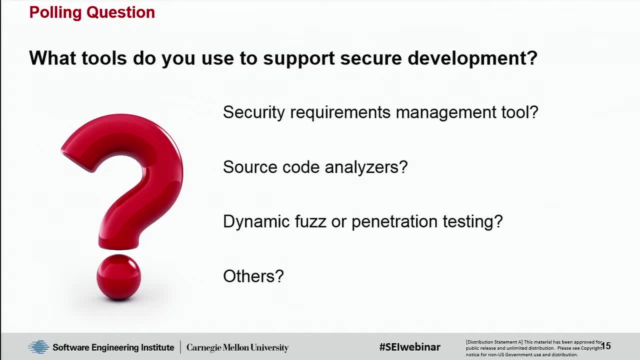 So the question you're going to see popping up now is: what tools do you use to support secure development, Security requirements management tool, source code analyzers, dynamic fuzz or pen testing or others? If you use multiple, feel free to type those into the Q&A box. 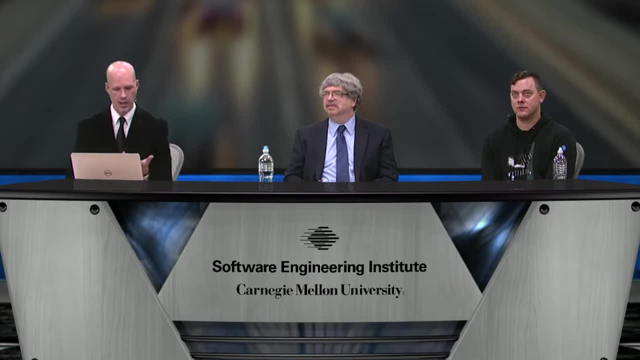 as we go along And while we give you about 15 or 20 seconds to vote there, we had some questions piling in for you guys, So maybe I'll address one to Chris here, from Brando asking: in your interaction with Jeep, did you? 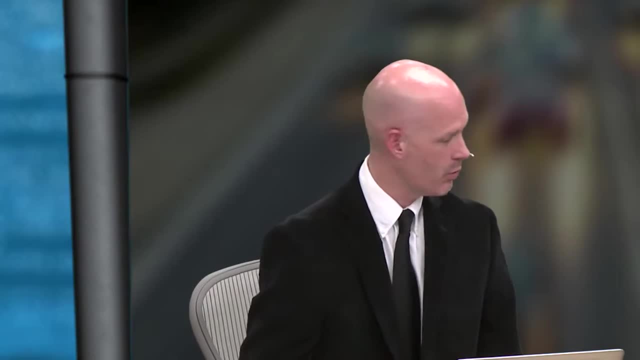 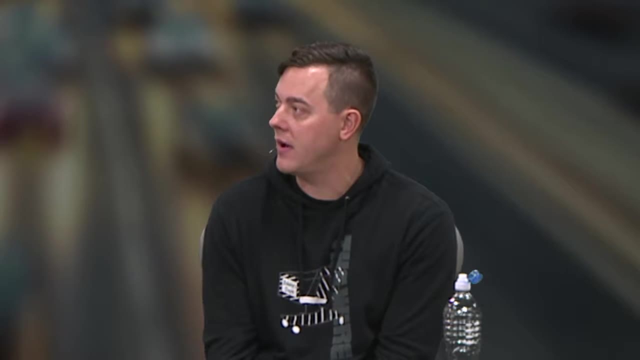 ask if they had done some type of security assessment or threat modeling. Yeah, I believe when we talked to them, they actually were aware of the vulnerability that we found And it was fixed in subsequent iterations of those vehicles. It just so happens that when you don't, have the ability to update over the air. it's hard to retroactively fix previous systems. So, like I said, they weren't completely blind. It's just starting. a security program takes time and it's going to be hard to fix everything backwards. 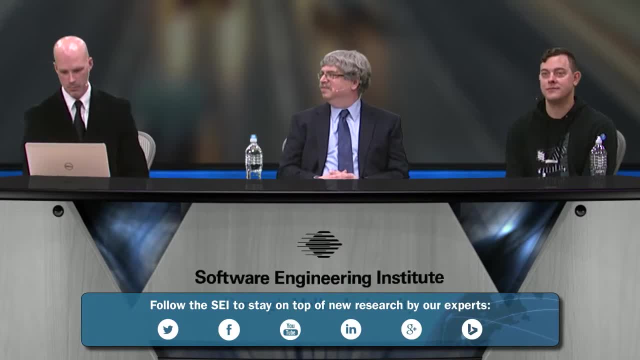 OK. well, this speaks into Brooke's comment. First of all she says: hi, Chris, You must know Brooke. But she says it sounds like a fairly complete failure to holistically threat model. You have to realize that these people are powerhouses. 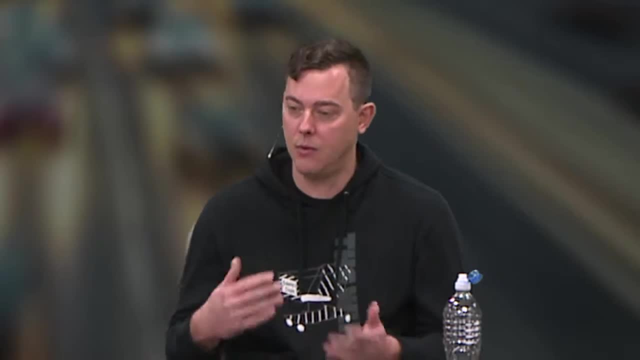 in engineering And you get in a car and it turns on every time And it works And you just have to change the oil and it'll run forever. But figuring out how to secure these things is hard to do And it's not an area of expertise. 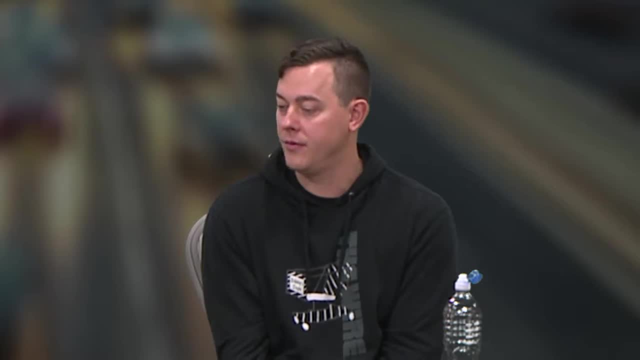 where there is as plentiful of skilled people to do so. So, while in retrospect it seems like it was a complete failure, I'm sure they were trying, But it's hard enough, I think, as everyone knows, to hire talented security people nonetheless. 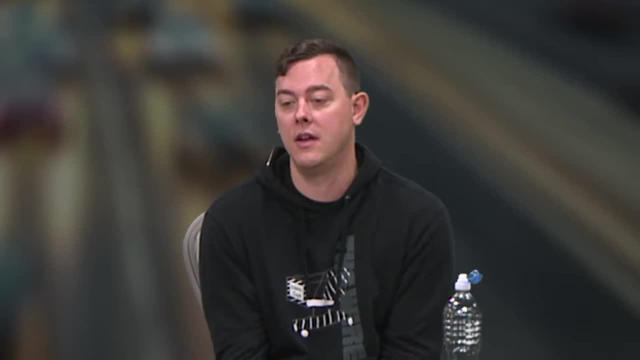 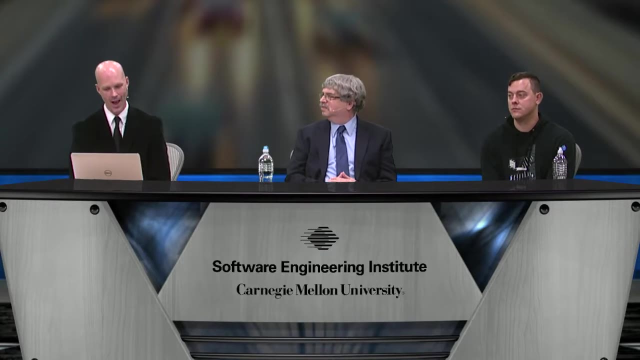 talented engineers. So really we're just hoping for the best And they can learn from it and move forward. And then we had a question from Ed asking any thoughts for an approach to permit self-hacking or extensions to firmware code. 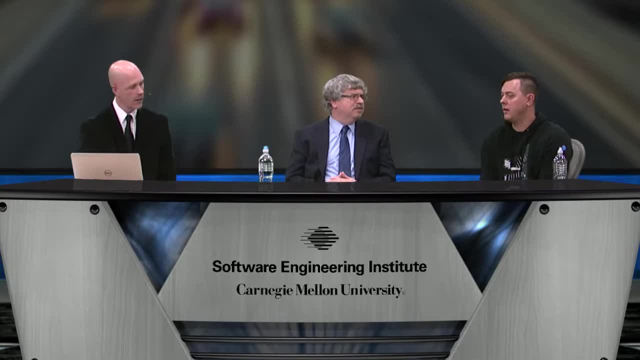 Maybe that's the both of you. I guess I don't understand One more time, Any thoughts for an approach to permit self-hacking Or extensions to firmware code? Oh, so I mean, if you want to hack the firmware and it's signed, then you won't be able to load it on the ECUs. Yeah, that's just a trade-off between having verified software and being able to tinker. There's the classic trade-off between flexibility and security. here, The ability to download your own code as a module into a system is a favorite way to extend the functionality for historically. 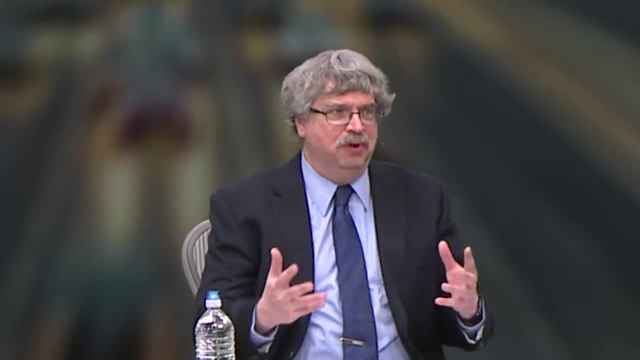 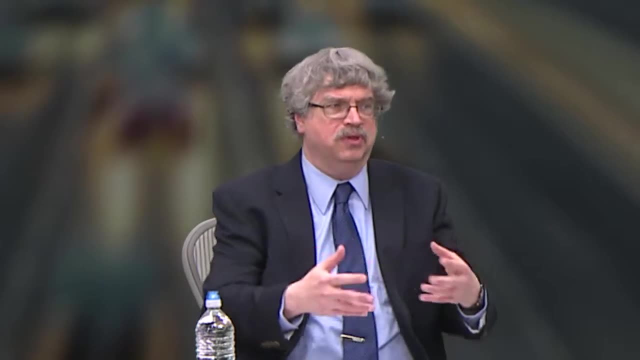 in the whole software world, But with it comes a whole slew of concerns about the things that we talked about, that you're operating in new environments. what kind of authentication is necessary? what authorization? how do you know where it's worth? how do you back it out? 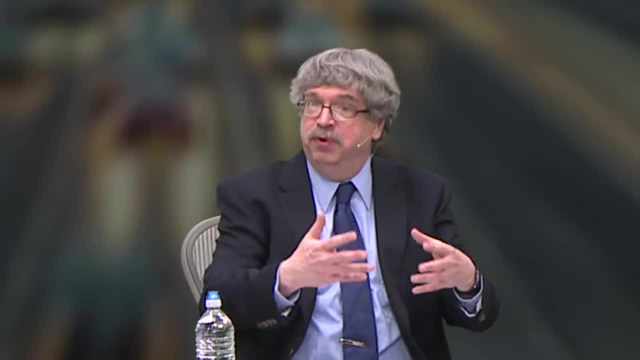 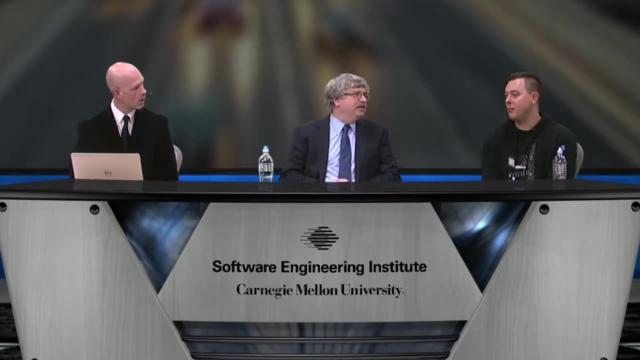 Most of the times, if you have a system that's high risk of causing physical damage, you want to be really, really careful about those kinds of things. Yeah, Unfortunately, I think people forget how much testing is done for the most minute code. 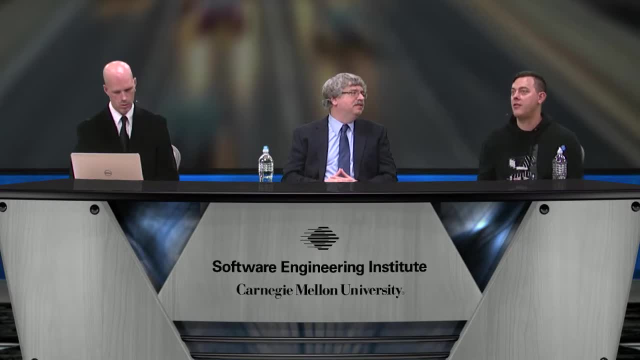 changes on these cyber-physical systems. Yeah, Yeah, So just changing itself might have an adverse effect to something else. That being said, I like doing it, But I understand why you might not want it to happen, Right, So I'll just wrap up the polling question real quick. 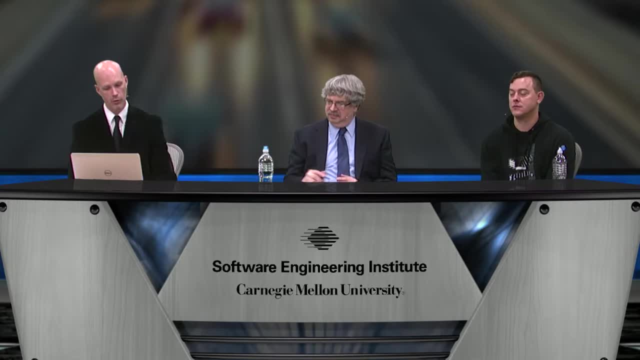 We had 19%. use a security requirements management tool: 41%. use source code analyzers: 19%. dynamic fuzz or pen testing and other at 22%. So back to Mark. We've got about 10 minutes left with you guys so we can go. 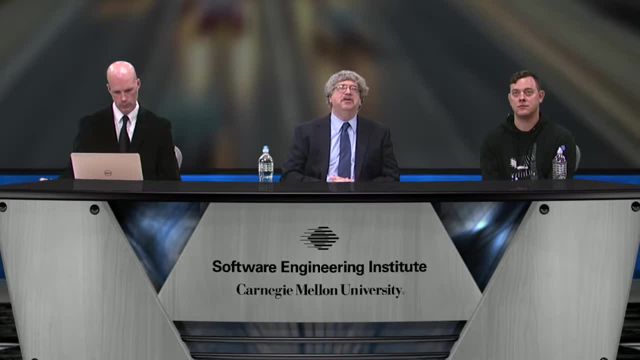 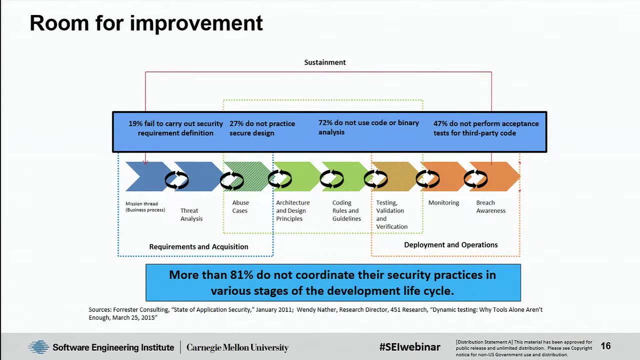 Sure. So just for what it's worth, here's some industry studies that have been done on these kinds of things And it turns out that about a fifth don't do any kind of requirements analysis in the security area. So it sounds like that we may be in the same kind of ballpark. 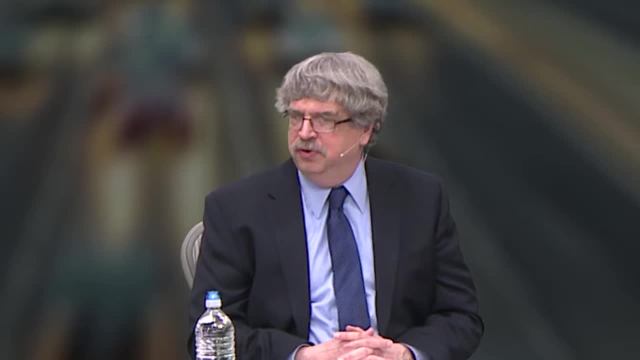 here A third really don't look to security issues in doing design and architecture. Surprisingly, nearly 3 quarters don't do any testing of security. Now, they do lots of other testing, a lot of functional testing, but actually doing static code analysis or fuzzing. 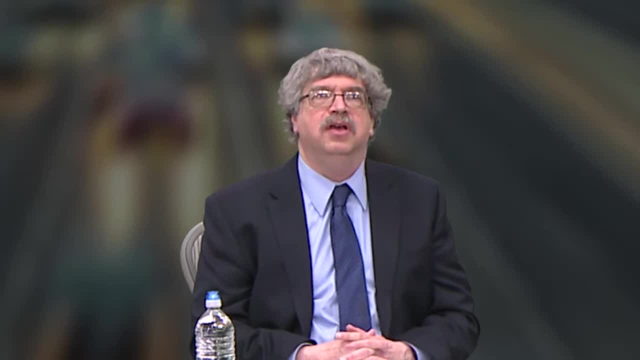 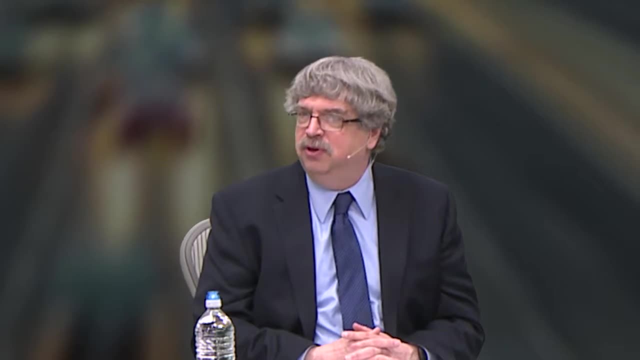 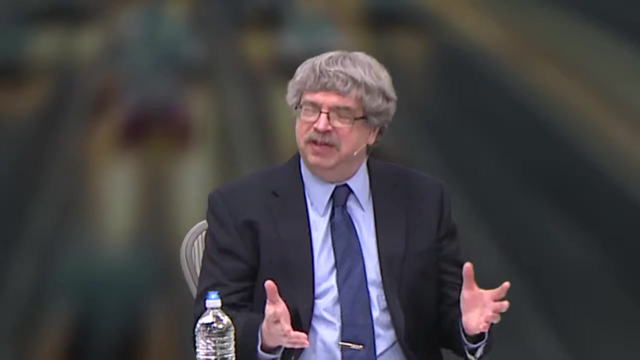 or things of that sort. to see whether you have security issues is not well practiced, And especially in these kinds of systems where you have a lot of third party components. nearly half don't actually consider the security issues of those components And perhaps more starkly, almost 80% or more. 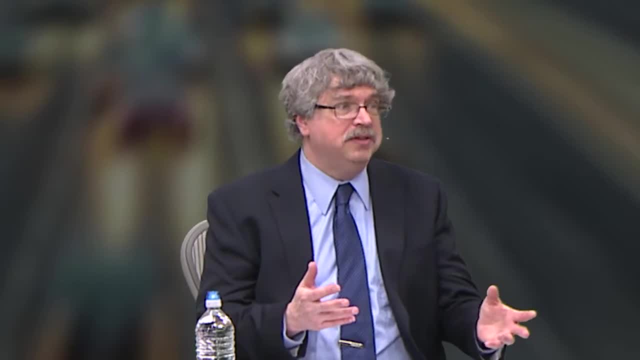 don't integrate whatever these things are across. So even if you have someone looking at the threats, that's not passed on to the people doing the design And, as a result, they're not designing against them, They're designing against those threats. 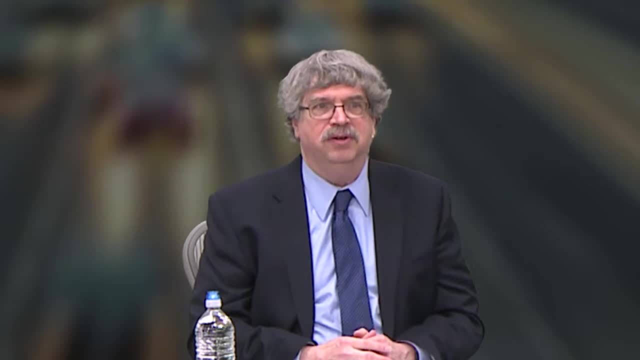 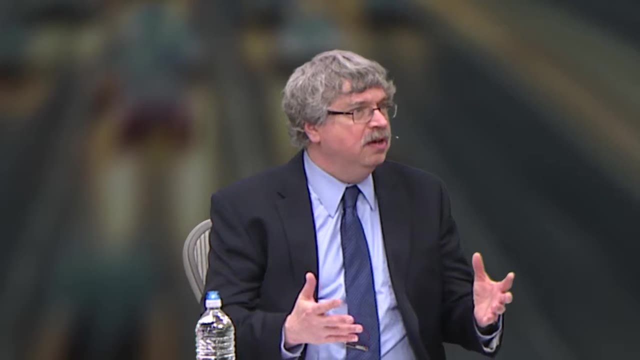 So you have a lack of communication, which makes this very hard to implement. But again, we know better And the point is by having this knowledge spread more broadly we can make these systems better without having to do a lot of new invention. 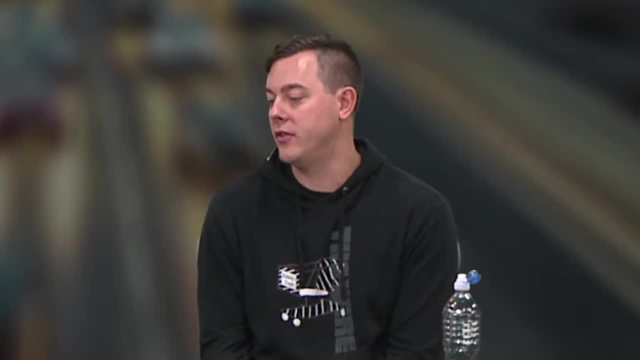 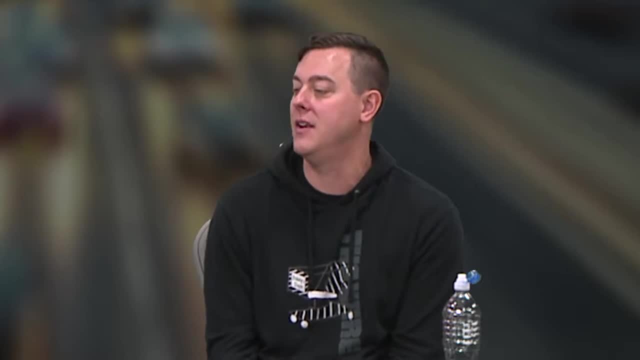 Right, Right, But to deploy signed code you have to have some kind of key management and self-signing service to make sure that the developer's code can actually be tested and run. So it really does bring up complications And I understand that. 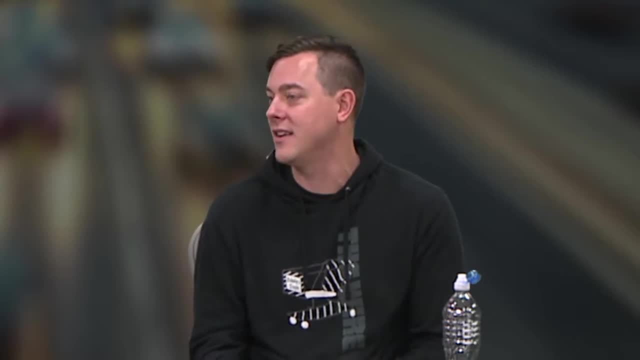 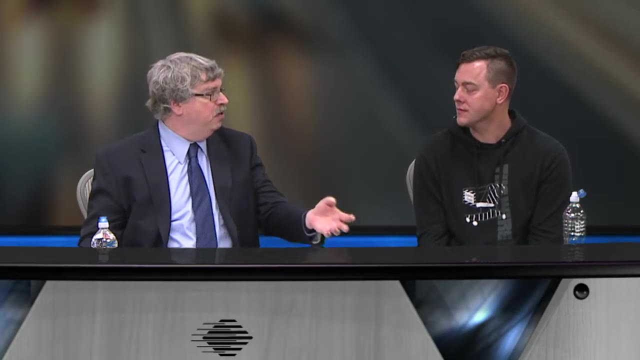 But at the same time you want to build these in to your model instead of trying to bolt it all on at the end, Right? So if you understand upfront that one of the threats is someone changing code or having doctored code coming into the system as one of the threats, 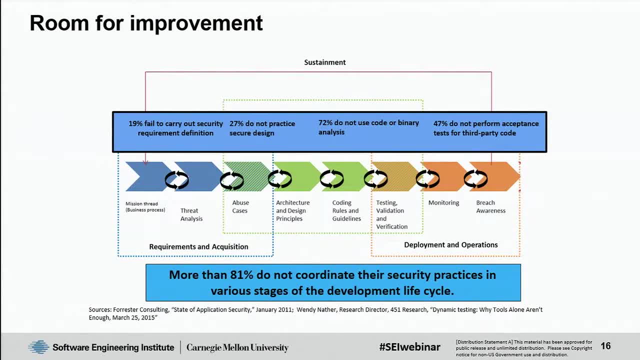 and one of the requirements, then it's going to be really difficult to figure out who's going to do it, Because obviously it's going to be a lot of data, And so you want to be able to figure out how you're going to do that. 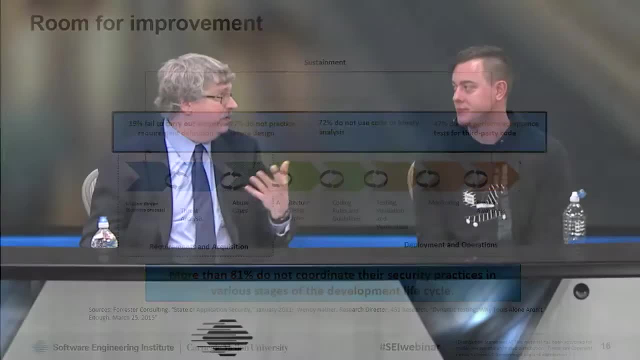 That's what you're going to be able to do, But you need to be able to do it by the time you get it done, because, at the end of the day, you're going to be able to do it by the time you get it done. 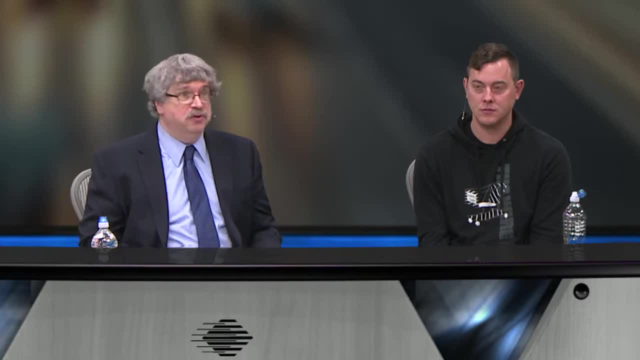 And that's where the data starts being taken into account all the way down the stream. So it's not, as you said, an add on at the end and we're saying, oops, we no longer know how we can do testing. 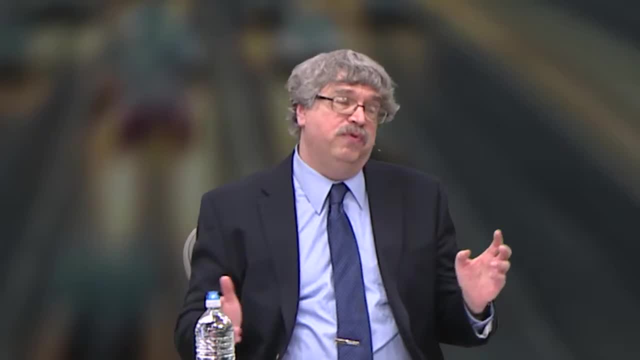 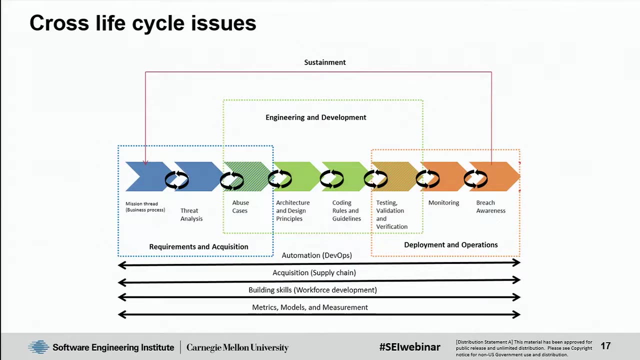 We no longer have a way to have our field service do updates. Yeah, And you don't know how to take away certificates and all the other issues are. In addition, we've mentioned a couple of times the assembly of these systems from third-party. 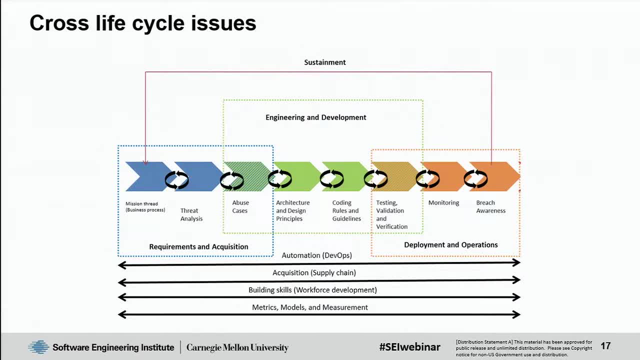 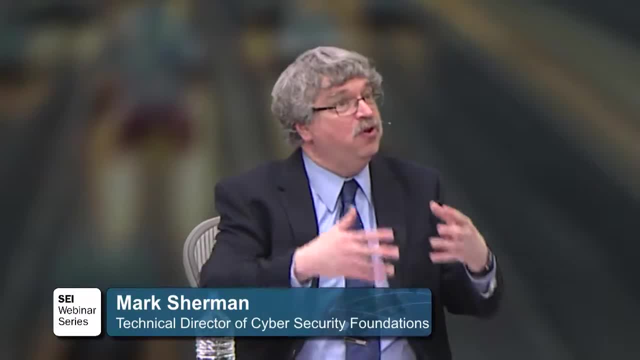 components, That's managing the whole supply chain. Fiat was on the front end. Well, in most cases, people tend to think of that final integrator as responsible for everything, even though it may have been a harming issue. The same thing with airplanes: It's United Airlines that's on the 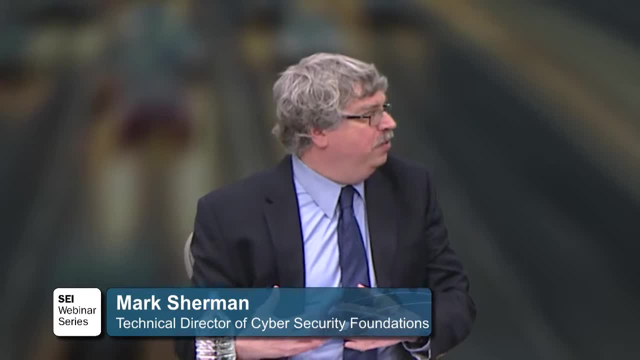 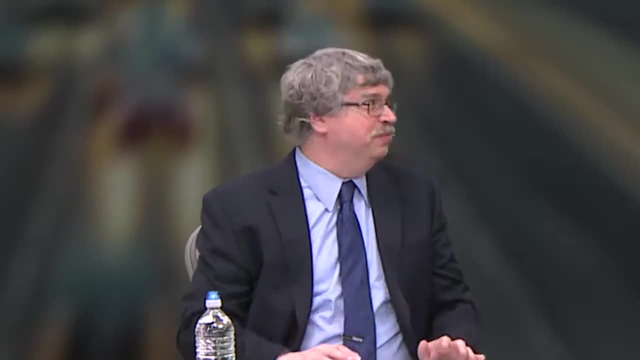 front end, and then it's Airbus, and then it's whoever provided the stuff to Airbus all the way back. But if a United plane falls out of the sky, it's United who's on the hook, not Boeing as the first place or whoever. Sorry, I don't mean to say nasty things about Boeing As you. 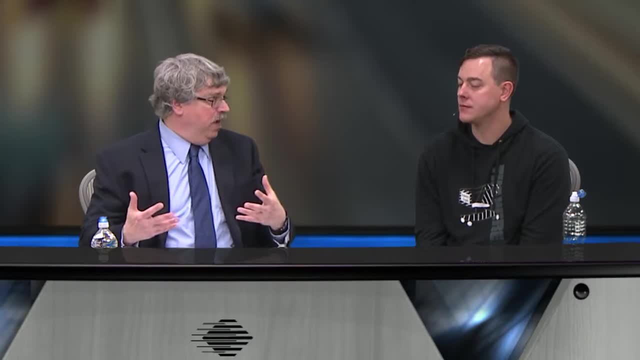 mentioned, there needs to be education. People need to understand what's going on. In some cases you can have a Bill Gates- tell the organization you shall do this- But in many cases this is more ongoing professional development throughout the whole development process And you need to. just keep track of things. You actually need to measure to see if you're getting anything right. You need to measure to see if you're getting anything right And you need to measure to see if you're getting anything right. And you need to measure to see if you're getting. 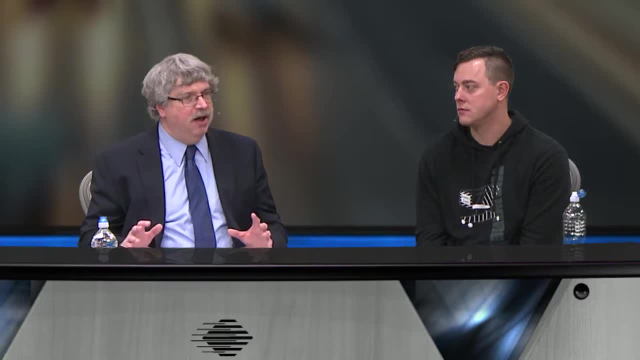 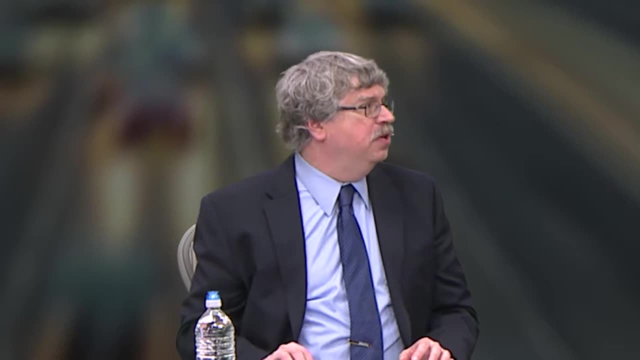 any better, And putting that in place so that you can keep track of not just defects and quality- which people have already done- but security issues as well, to make sure that, in fact, you've got something that's improving over time. So with that we can start to move into the 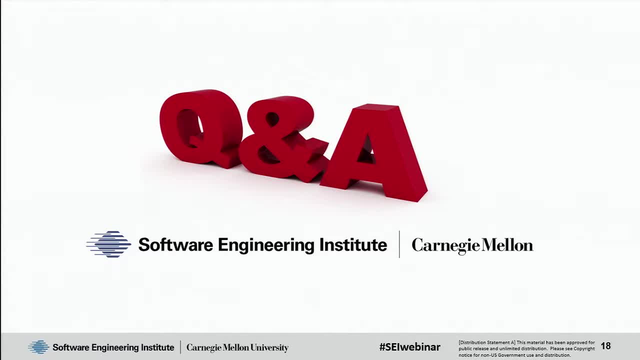 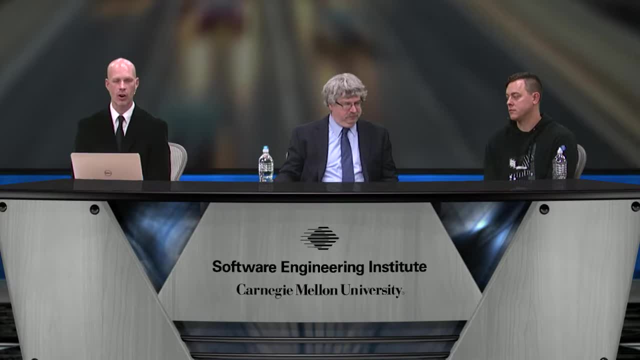 actual discussions on some of the individual pieces. Did you want to? Great? So we're getting some audience questions. We're getting a number of questions asking if an archive or the slides are available. Every presentation today is being archived. folks, It's the same registration you. 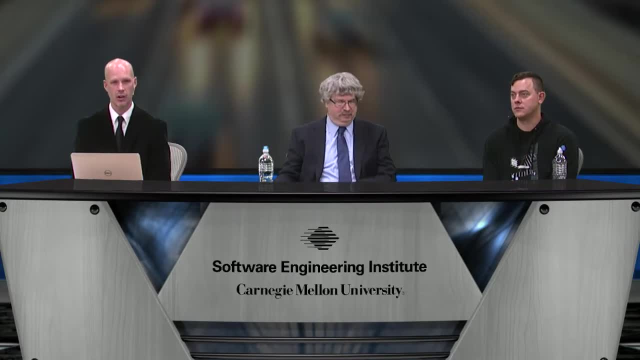 can access. It's the same URL that you got to log in today. You can access it. Most likely the archive will be up by tomorrow and you can catch the archive version. As for slides and materials, if you look in the Download Materials tab at the bottom of your console, you'll see a link to walk. 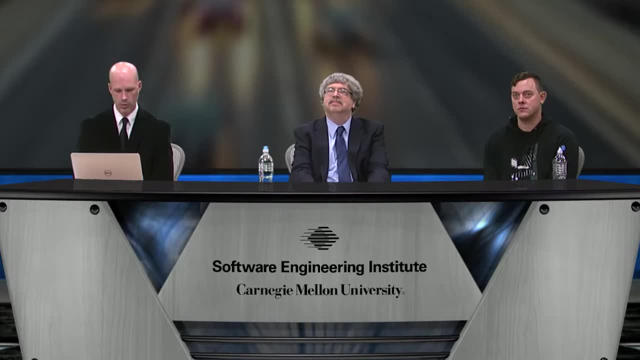 away with those slides now. So just a couple more, a little bit more time with Chris and Mark here. So, Mark, when you started at the beginning, you talked about a Department of Transportation study. Do you have a link that we can share with the audience, or can we send that after the webinar? 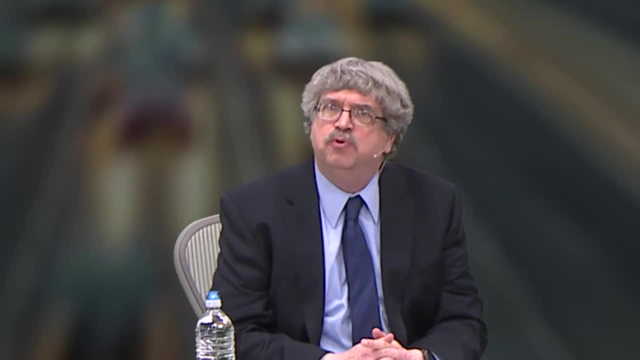 that people can access After the webinar. As I was thinking about it, I heard that there was a. this was referred to me from the Department of Transportation. I'm actually not sure that they did the study as opposed to refer to the study, but I do have the link, Okay, so we'll get that. 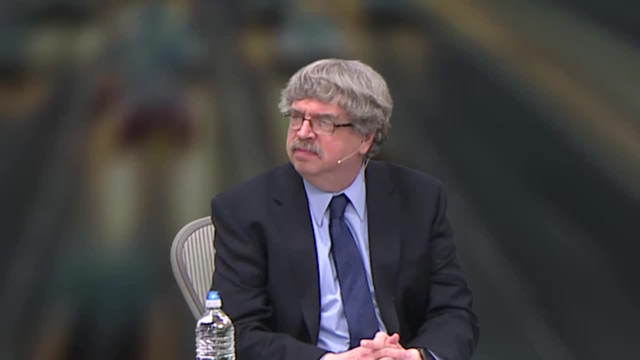 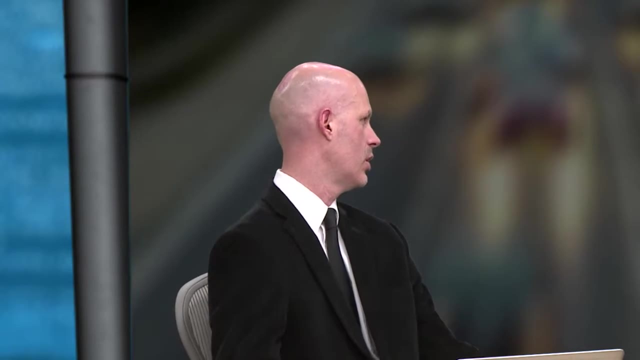 out or we'll add it into the resource sections. Brooke wants to know: do you know if they met MISRA in their code And the comment says not that this would help design issues? Yeah, I have no clue. You know, we never actually saw source code other than some scripts. The rest was just binary format. 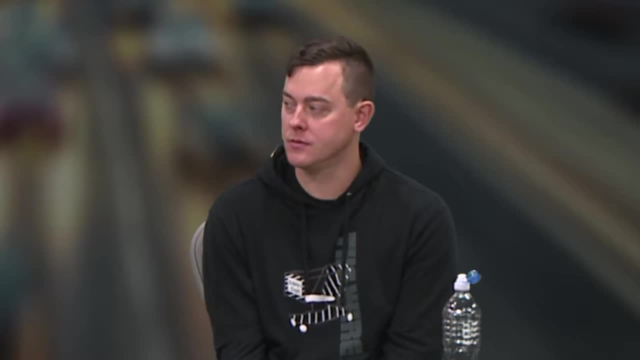 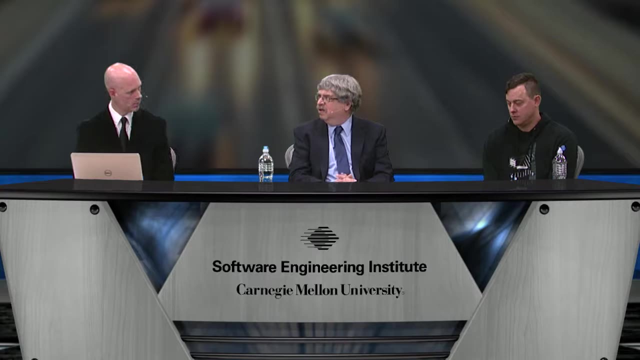 so we wouldn't be able to say Okay from Brando asking: can you address some of the best practices to manage risk When integrating that ecosystem you talked about? And we'll add both of you. So actually there's the reason why I'm hesitating. I'm trying to figure out how much is going to be discussed. 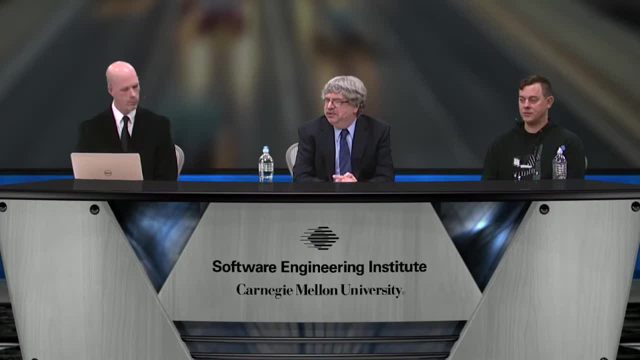 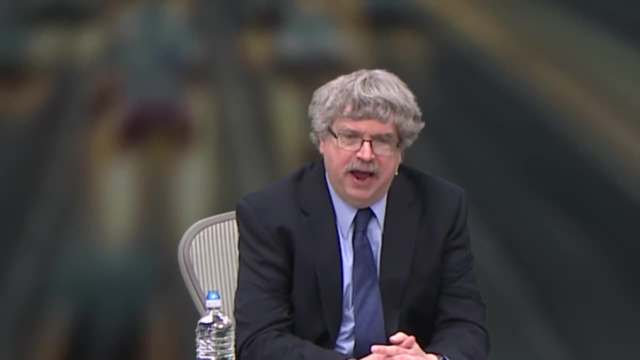 later. I know that some of the other speakers are going to address some of those issues. So there's a general methodology where you look at the supplier, the product, the distribution and the operational environments in order to evaluate third-party components. Supplier. 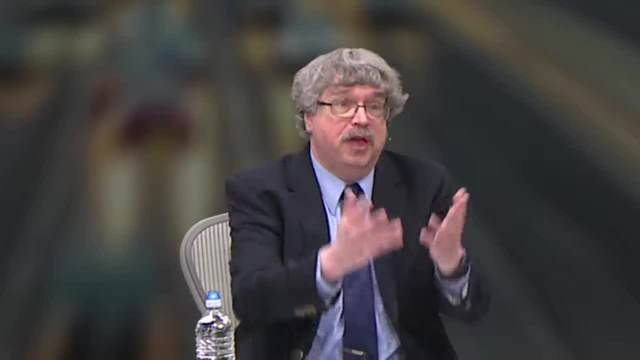 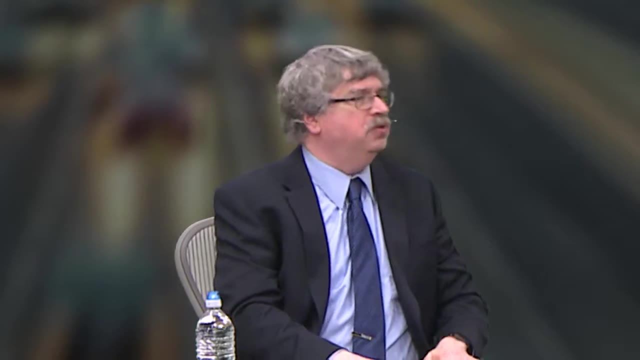 are they well equipped to build secure software? Do they know things like a secure software development environment, maybe threat analysis, things of that sort? The product: is it signed? Is it built? Has someone actually validated? Have they done static testing on it? Have they done? 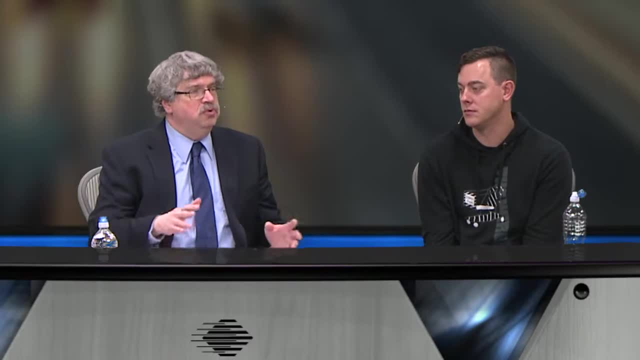 penetration, testing on it or not? Distribution channels: do you know that the code has reliably made its way from the source to wherever it's going to be installed? Do they have an over-the-air kind of thing? How quickly can things be addressed? And the operational environment which is 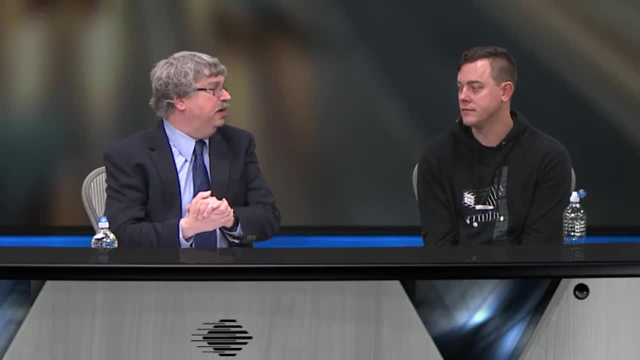 what assumptions have been made? Am I assuming that I'm not going to be connected to the internet? I only have physical access? Or have I taken into account that I'm going to be in this open kind of an environment and this thing changed? Those are the general 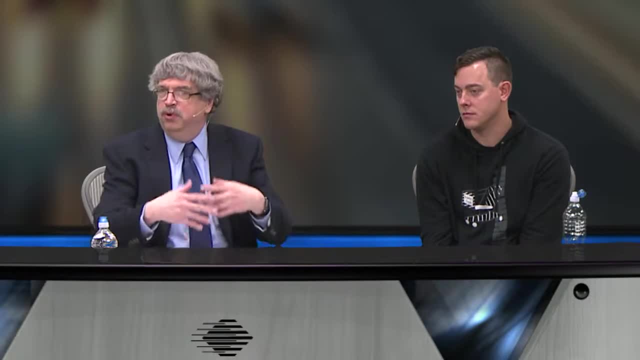 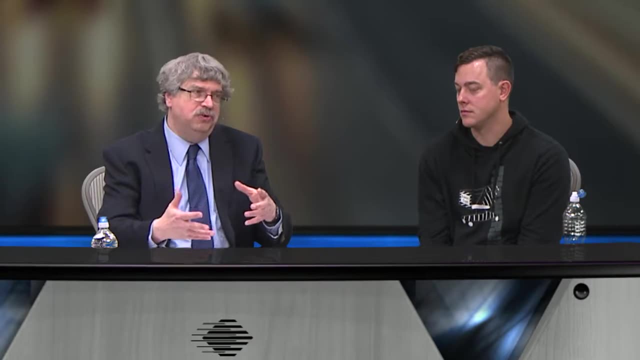 kinds of thoughts one does in general with third-party components. When you get into open source, there's more issues about provenance and making sure that you have a catalog of what components you're using and how to find them later when you need to update them. So 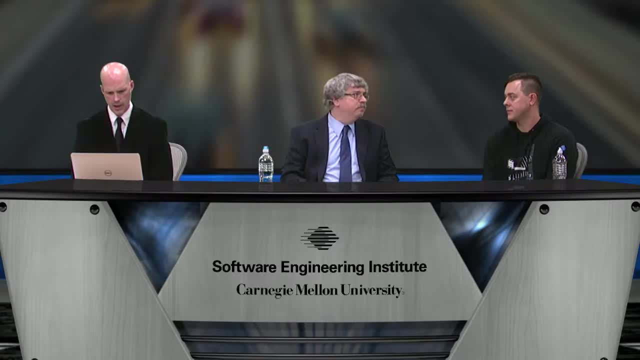 there's actually a lot of material that's been written up about this Terrific And just the last one in the queue here asking more. I think you mentioned a figure of hundreds of millions, Millions of dollars. Neil wants to know: do you have a? where did the figure? hundreds of millions? of dollars to correct the issue come from So hundreds of millions of dollars that FCA was affected that they had to set aside in order to do the recalls. And I have the. I don't recall whether it was in an SEC filing or something of that sort, but I can also give you the reference. 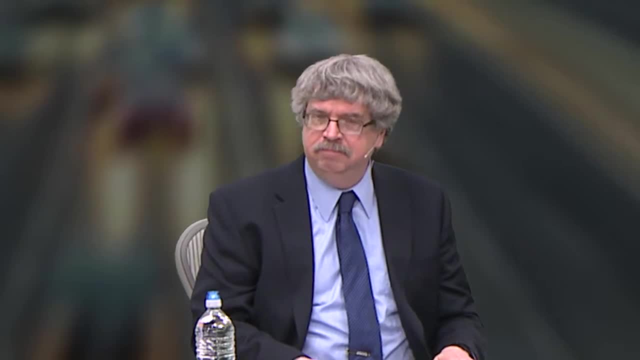 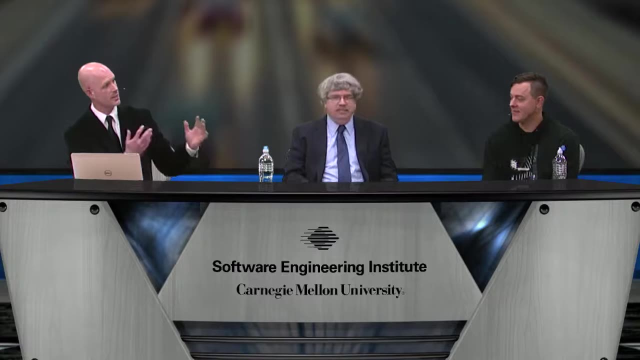 for that as well later. Okay, So that the queue's now empty. We're running a little bit ahead of schedule, So we're going to prepare for our next talk. I just want to thank Chris again for participation today. Anything you want to say about SummerCon, We know that's your conference. 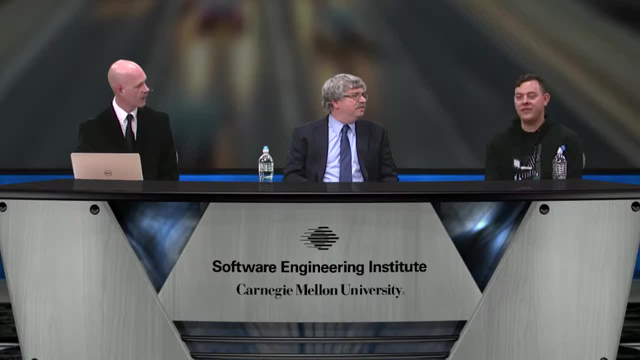 coming up. Yeah, it'll be in New York in July. Go on there 15th and 16th, head on up. It's a good time, Mark. thank you again. Excellent presentation. Any closing comments before we welcome in Chris. 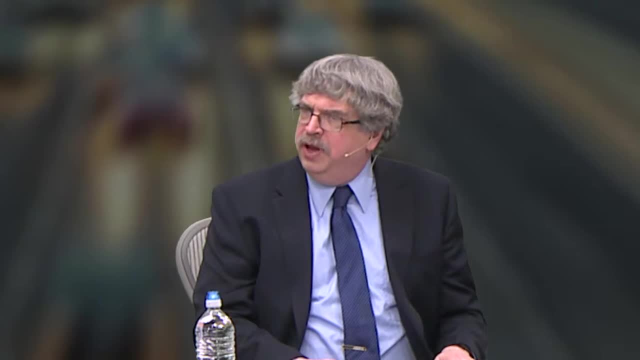 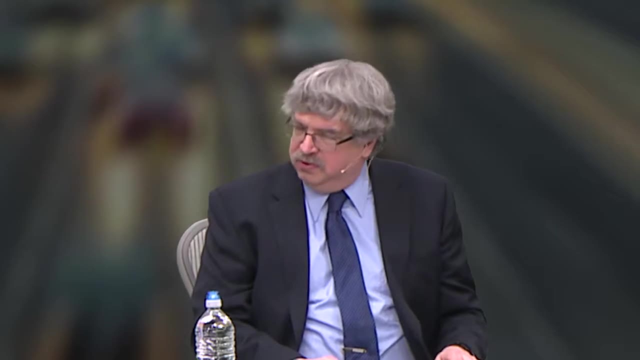 Just a plug, if you like. Sure, We have put together a white paper on cybersecurity for these kinds of systems in the automotive space And that is actually in the downloads. So that's one of the downloads And I know that the reference in particular for the Chrysler comment. is in that paper as well. 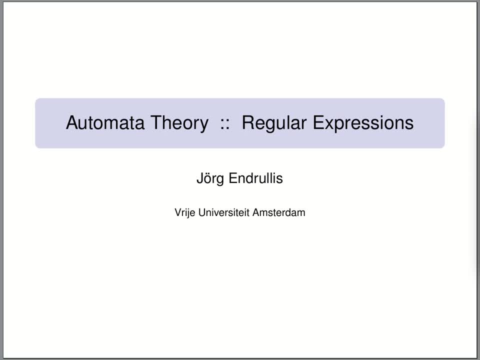 We've learned that regular languages can be defined via finite automata, via regular grammars. A particular popular way to define regular languages are regular expressions. They are heavily used in programming languages or in system tools such as grep or sed in linux, And they are used a lot in order to extract information, to extract certain pattern.